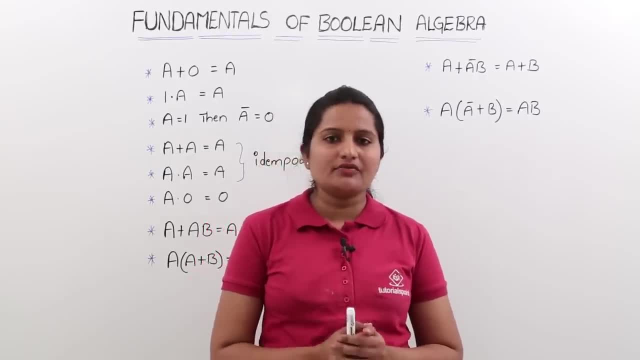 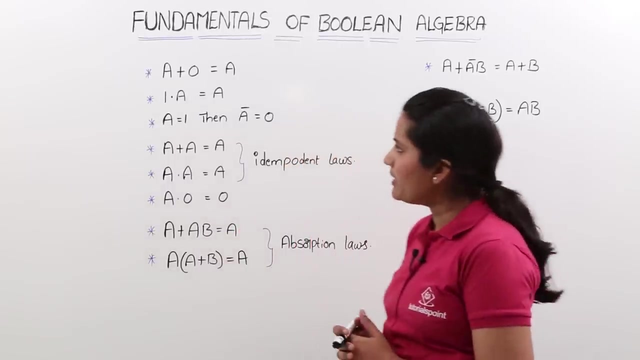 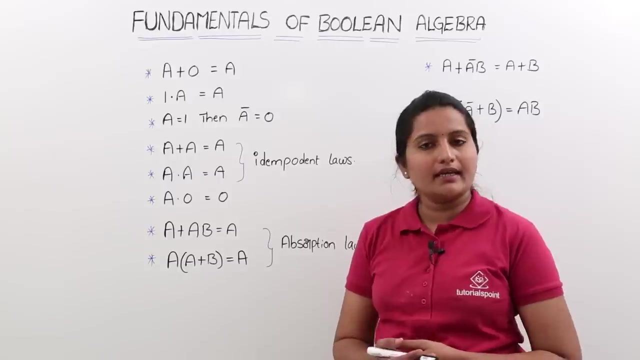 In this class we are going to discuss about fundamentals of Boolean algebra. These fundamentals are very, very important when we are solving Boolean expressions. To solve any Boolean expression, we need to apply this fundamental to get the answer easily. So see the fundamentals of Boolean algebra here. First one is a plus 0. is there? then we can take it. 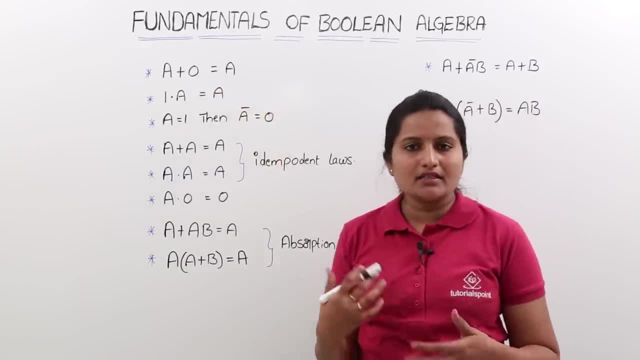 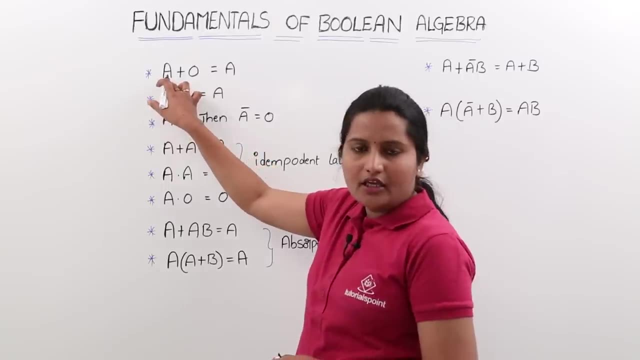 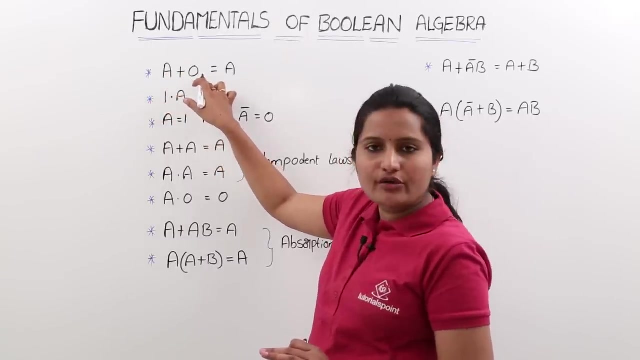 as a. a plus 0 is equal to a, Why we are taking a plus 0 as a means, For example, in case of a, if you are representing that as 1.. For example, a is equal to 1.. 1 plus 0 is equal. 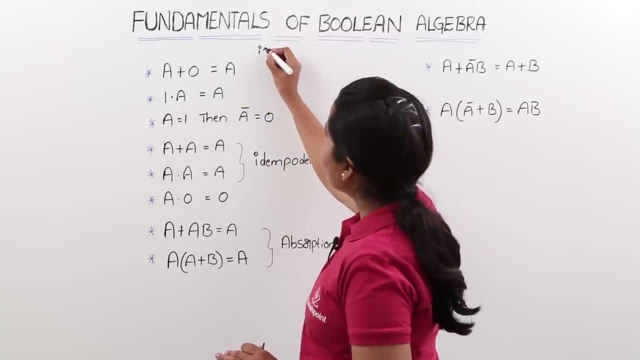 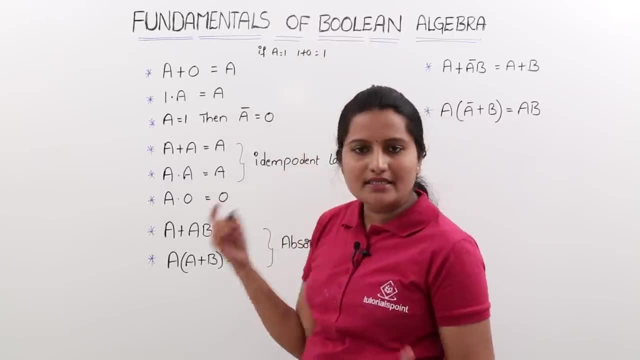 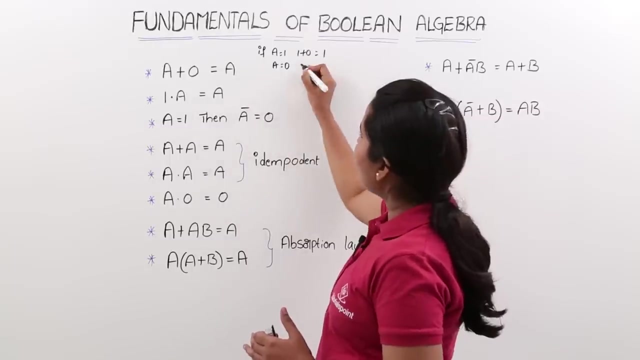 to 1 only. So that means, if a is equal to 1, then 1 plus 0 is equal to 1.. You are getting a only Whatever a is there. you are getting a a only. So, for example, a is equal to 0, then in a plus 0 plus 0, you are substituting, you are. 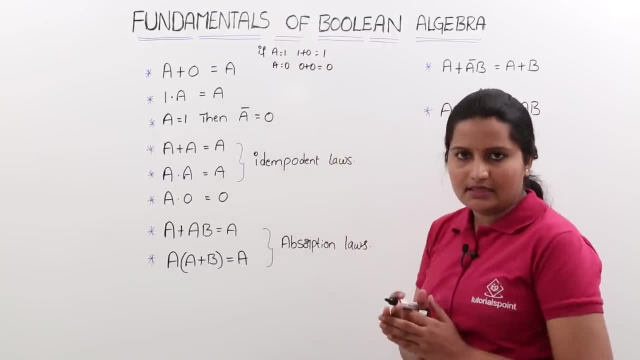 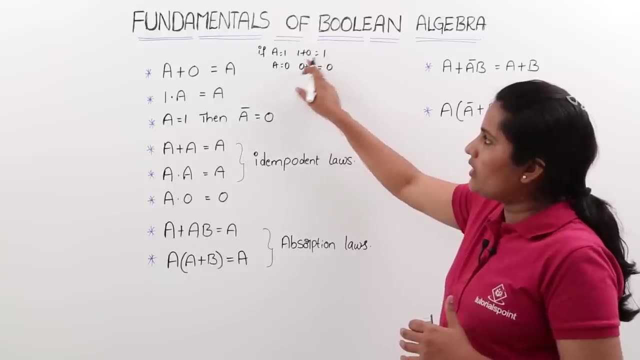 getting 0. So in these both cases, so a is having only two possibilities: either 1 or 0. If a is 1, again you are getting 1.. a is 0, that is 0. Whatever a you are taking, that is coming in the output. 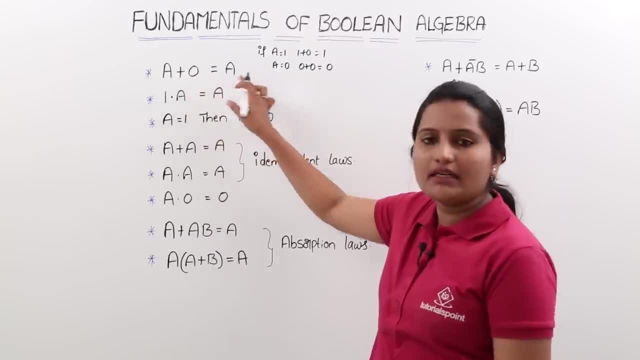 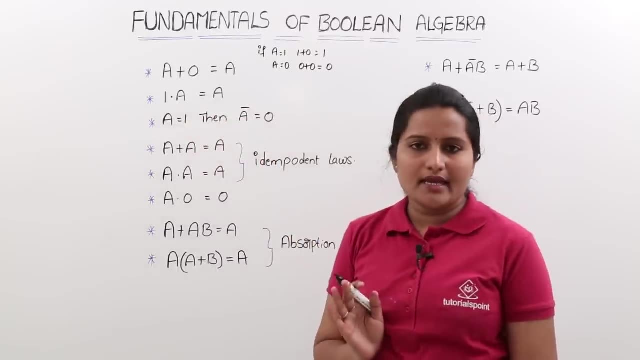 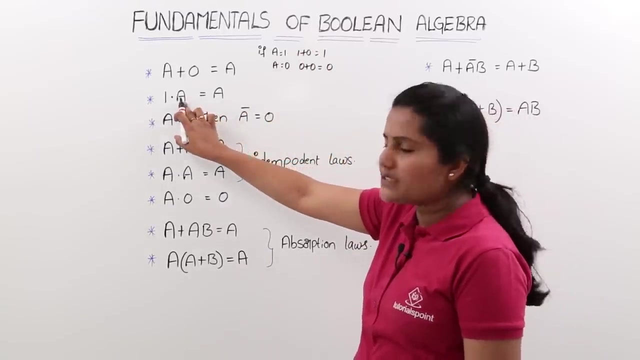 So that that is why a plus 0 is nothing but a. We can write like this: So now, 1 into a is equal to a, 1 into a is equal to a. This is also solved by using this theory. So that means, for example, a is. 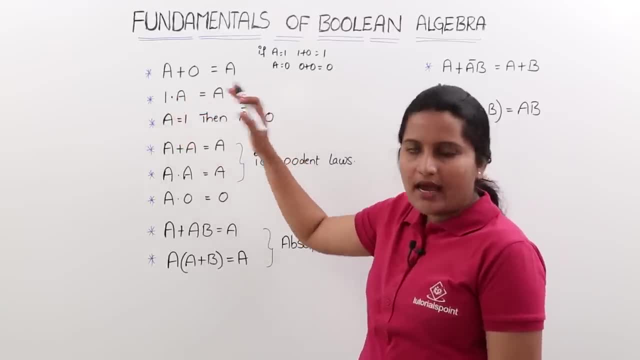 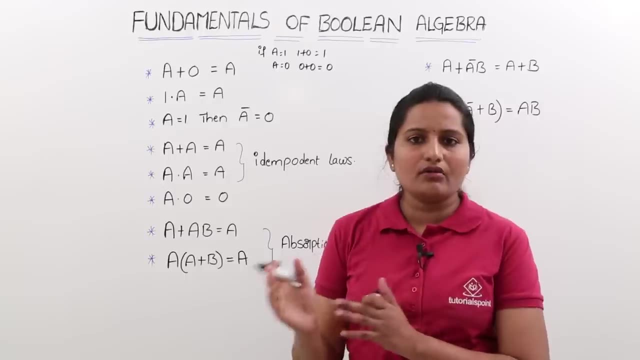 equal to 0, you are getting 1 into 0 as 0.. And for example, a is equal to 1.. 1 into 1, you are getting 1.. So, whatever a, you are considering that only, you are reflecting as 0.. 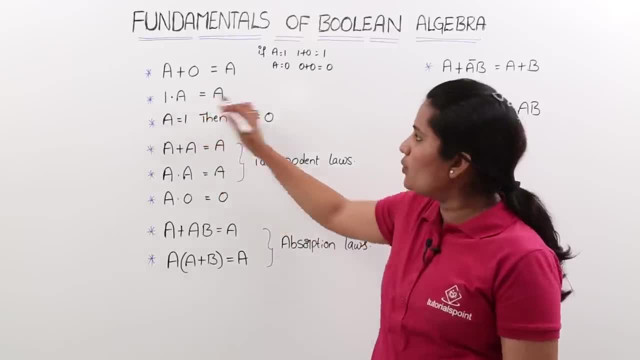 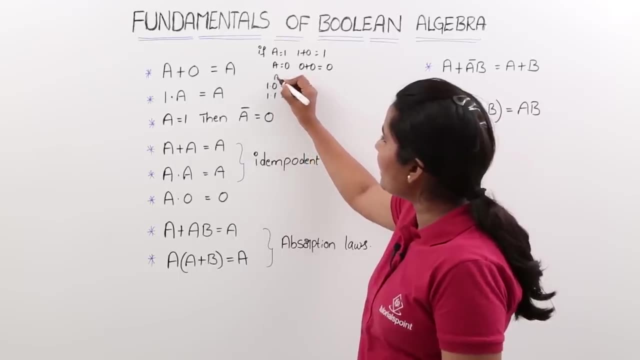 The result of this expression. So 1 into 1- that means 1 into 0- is equal to 0.. 1 into 1 is equal to 1.. These are the a values. If a you taken like 0, you are getting 0 only If you are taking a as. 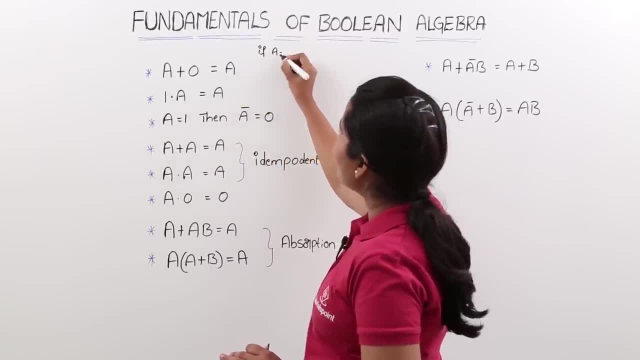 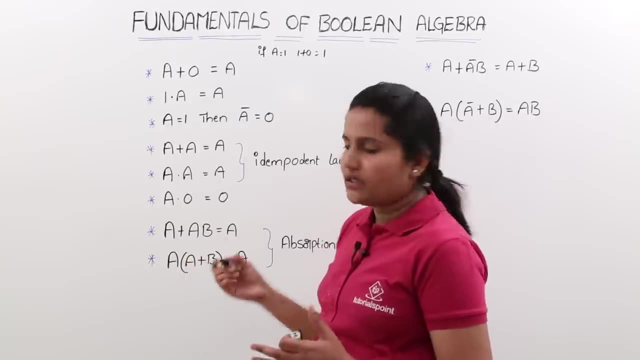 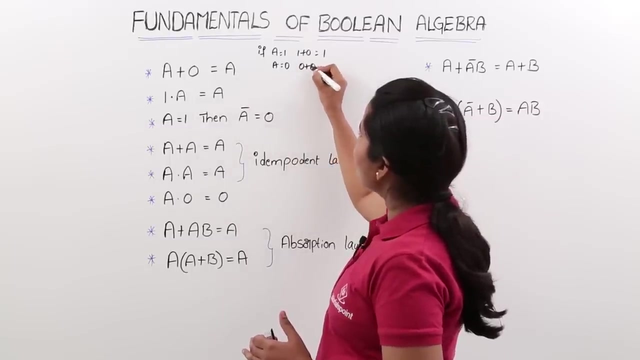 that means, if a is equal to 1, then 1 plus 0 is equal to 1.. You are getting a only. whatever a is there, you are getting a a only. So, for example, a is equal to 0, then in a plus 0 plus 0, you are substituting, you are. 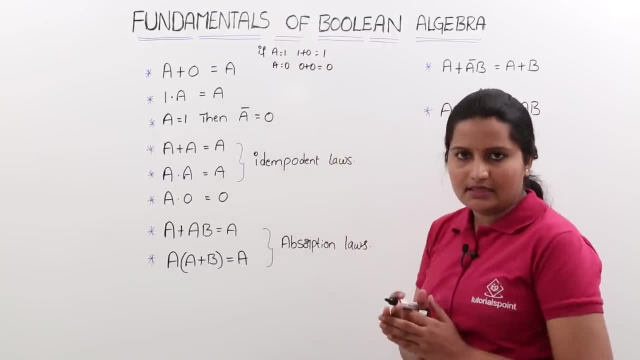 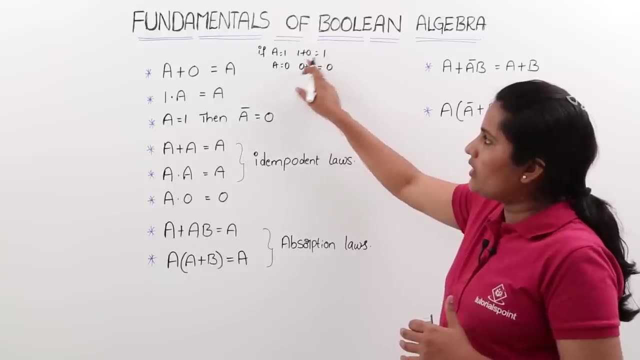 getting 0. So in these both cases, so a is having only two possibilities: either 1 or 0. If a is 1, again you are getting 1.. a is 0, that is 0. Whatever a you are taking, that is coming in the output. 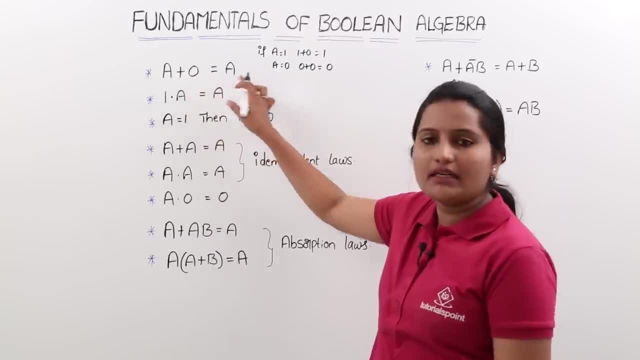 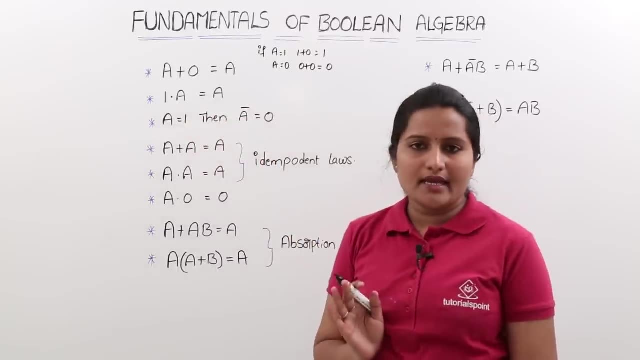 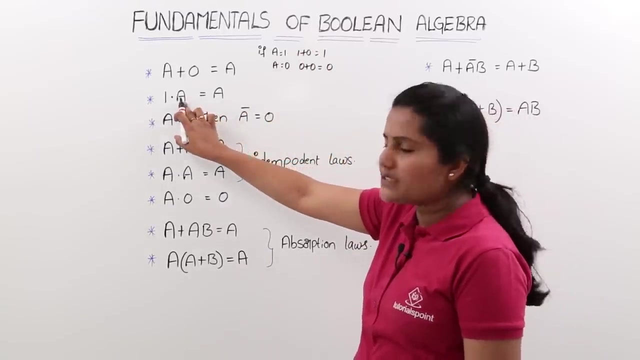 So that that is why a plus 0 is nothing but a. We can write like this: So now, 1 into a is equal to a, 1 into a is equal to a. This is also solved by using this theory. So that means, for example, a is. 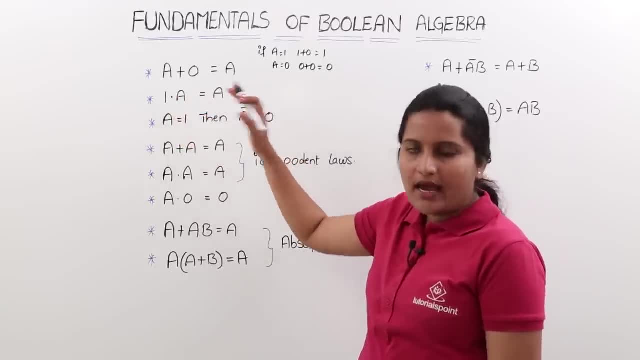 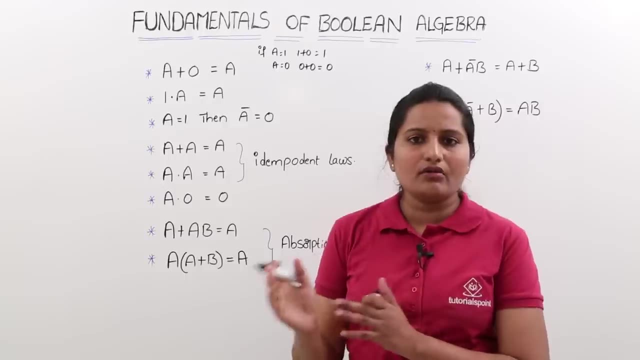 equal to 0, you are getting 1 into 0 as 0.. And for example, a is equal to 1.. 1 into 1, you are getting 1.. So, whatever a, you are considering that only, you are reflecting as 0.. 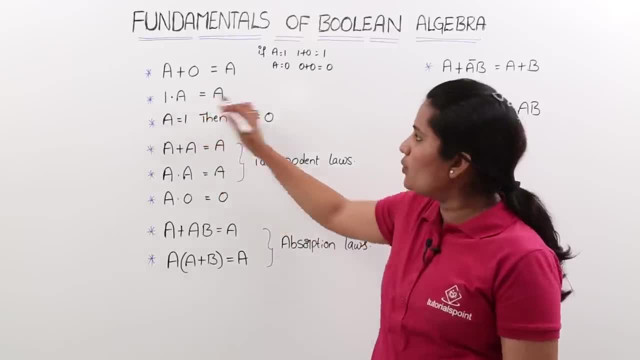 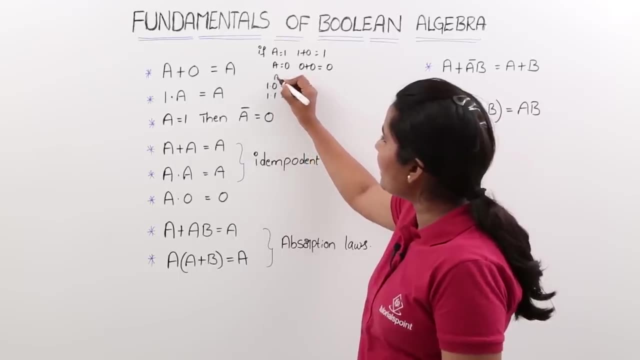 The result of this expression. So 1 into 1- that means 1 into 0- is equal to 0.. 1 into 1 is equal to 1.. These are the a values. If a you taken like 0, you are getting 0 only If you are taking a as. 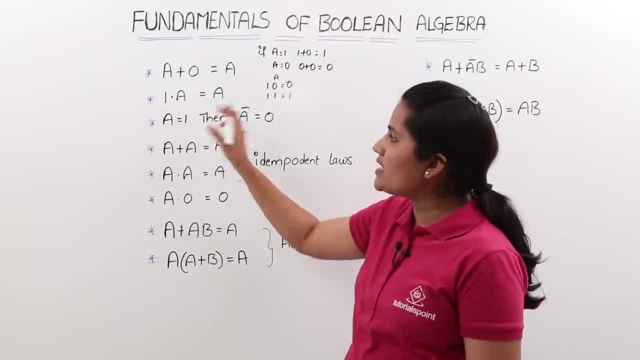 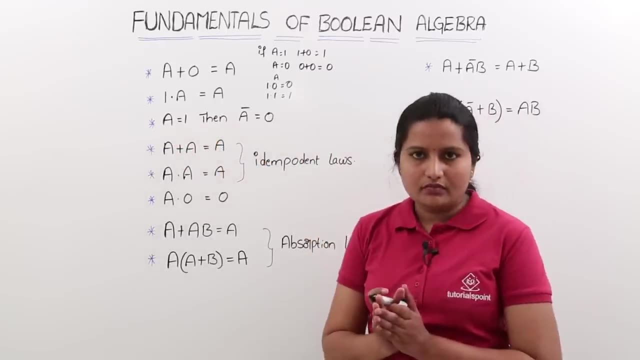 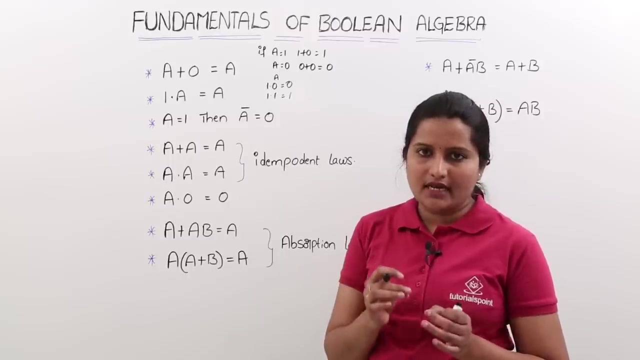 1, you are getting 1 only. So that is why 1 into a is also equal to a. So now a is equal to 1, then a bar equal to 0.. Always we know that complement Of anything is equivalent to its negative value. That means, for example, if you taken 1, the 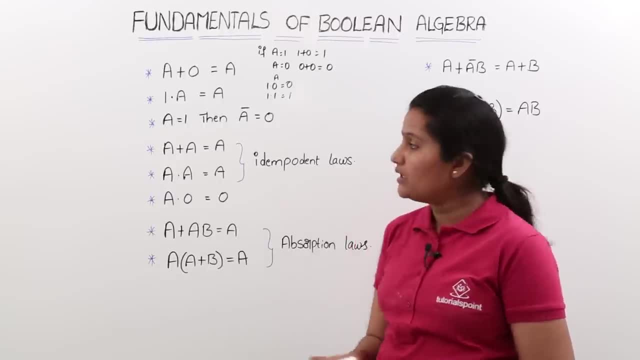 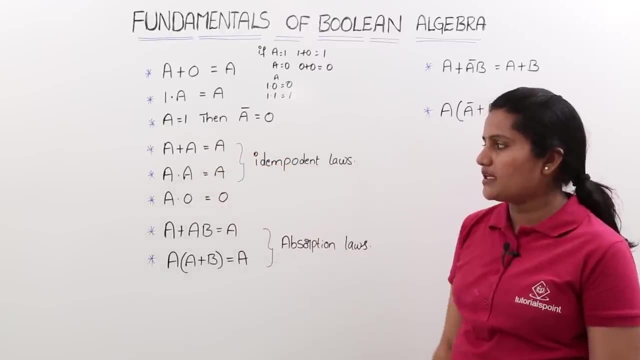 complement is 0.. If a is equal to 0, complement is 1.. So third property is: fourth property is a plus a is equal to a. Fifth is a into a is equal to a. These two are called as idempotent loss. 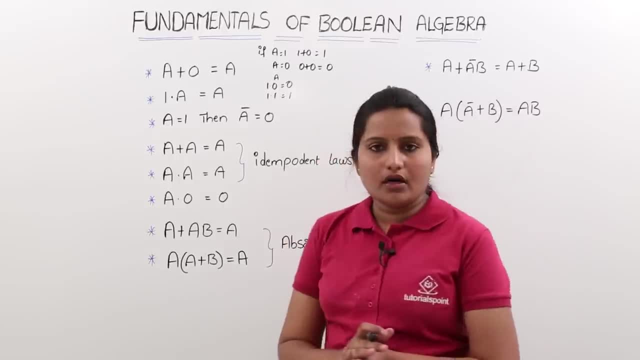 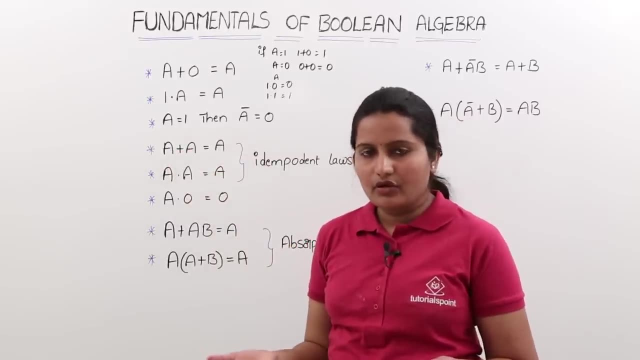 These are also called as idempotent loss. Now we are going to solve these two. also how we are getting a plus a is equal to a. We are. we know a plus a is equal to a, but how? So here to solve that. I am considering this here. 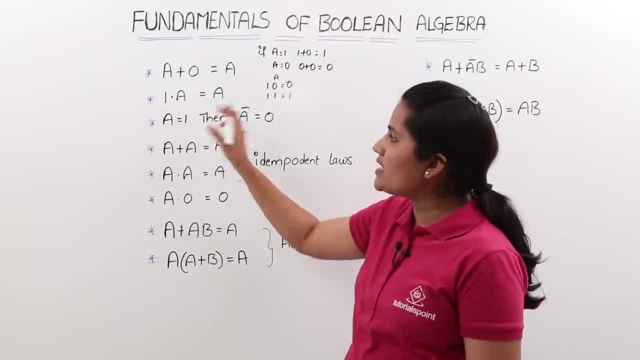 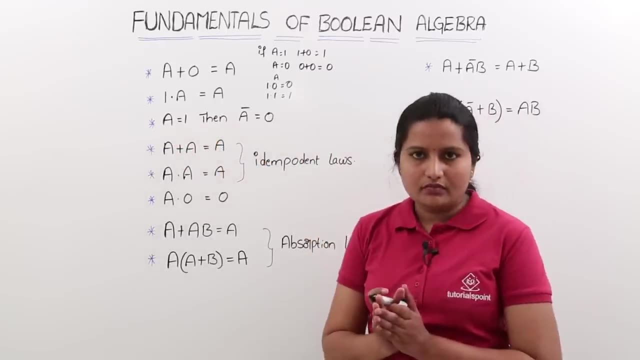 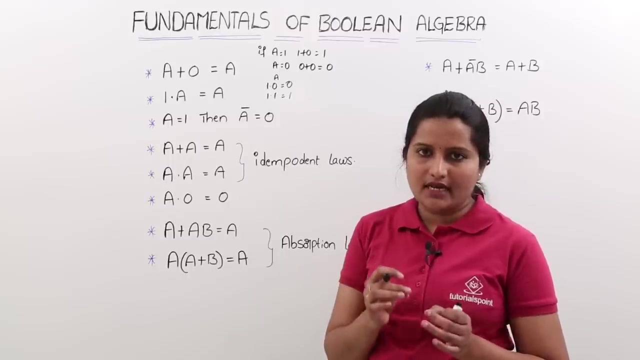 1, you are getting 1 only. So that is why 1 into a is also equal to a. So now a is equal to 1, then a bar equal to 0.. Always we know that complement Of anything is equivalent to its negative value. That means, for example, if you taken 1, the 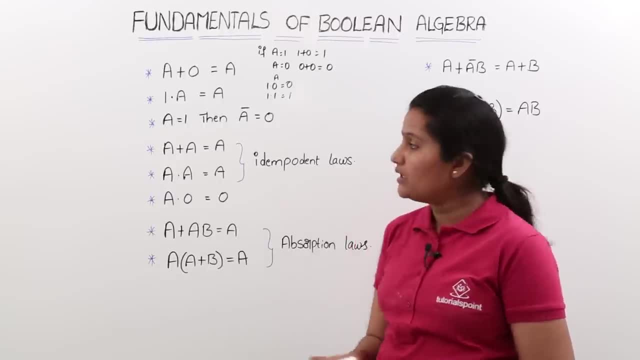 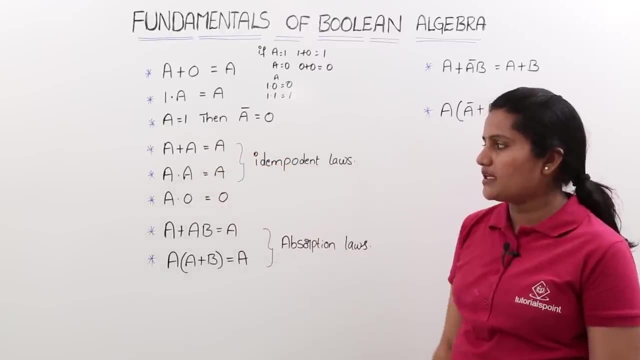 complement is 0.. If a is equal to 0, complement is 1.. So third property is: fourth property is a plus a is equal to a. Fifth is a into a is equal to a. These two are called as idempotent loss. 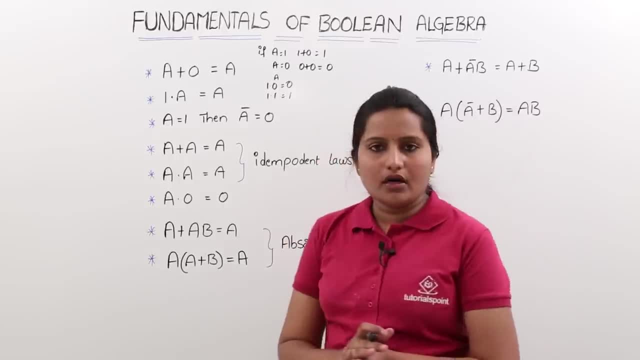 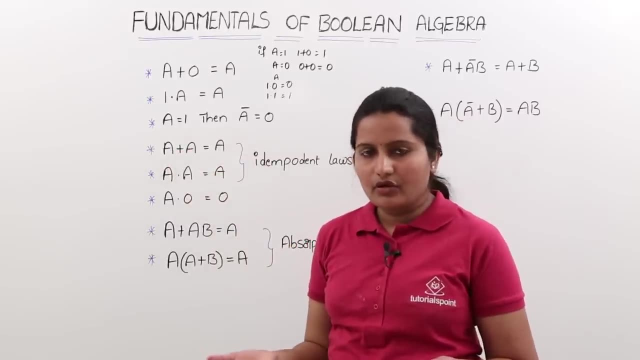 These are also called as idempotent loss. Now we are going to solve these two. also how we are getting a plus a is equal to a. We are. we know a plus a is equal to a, but how? So here to solve that. I am considering this here. 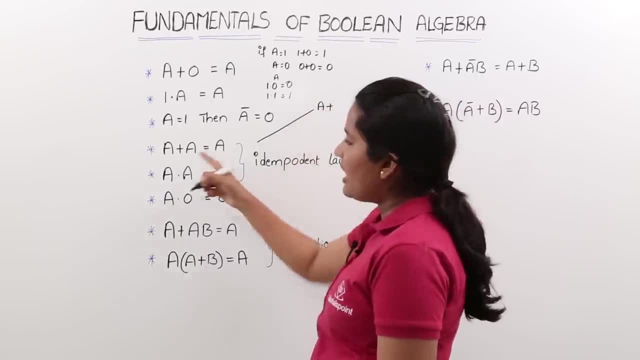 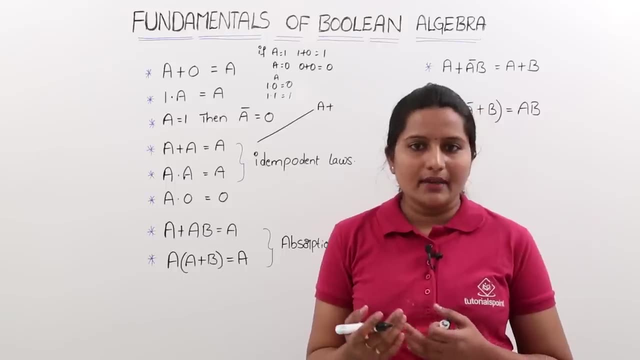 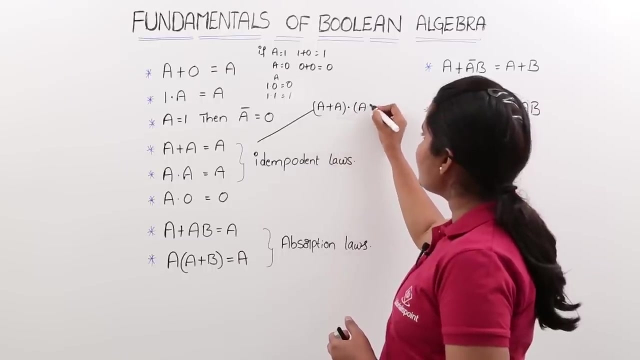 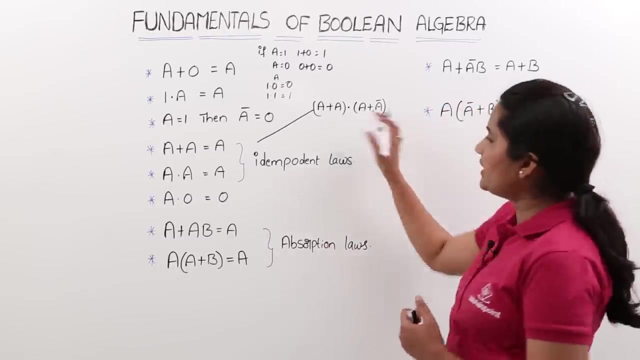 a plus for this a. I can take a plus a bar also. For example, if you are having a plus a here, I am just considering into 1.. Into 1 means a plus a bar I can take. a plus a bar is equal to 1.. Because so here a plus a bar means, for example, a is equal to 0, definitely a bar is. 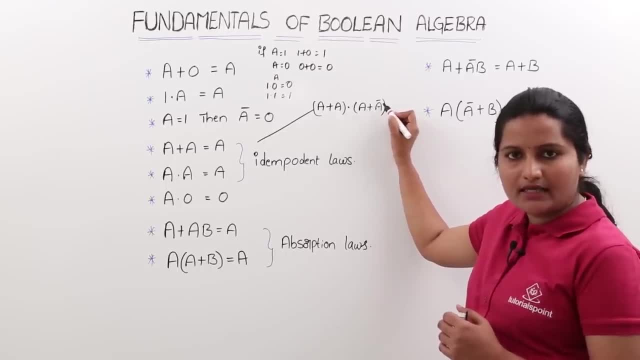 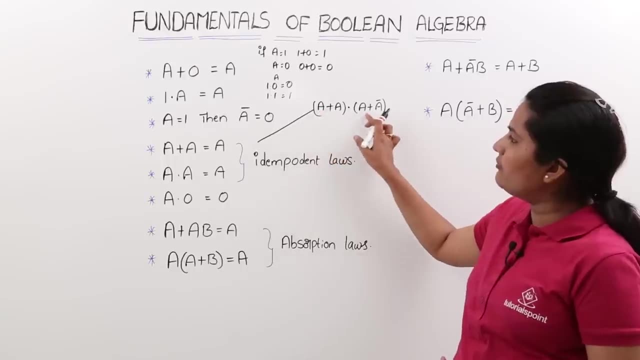 1.. If a bar is 1, if a is 1, a bar is 0.. In any case of a, the value is equal to 1.. So if I multiplied anything with 1, we are getting same thing by using this. So that is why I am just. 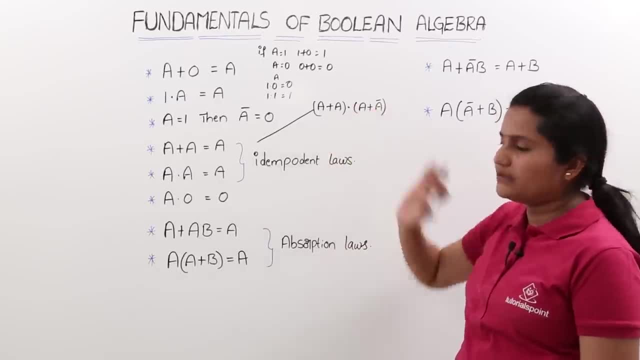 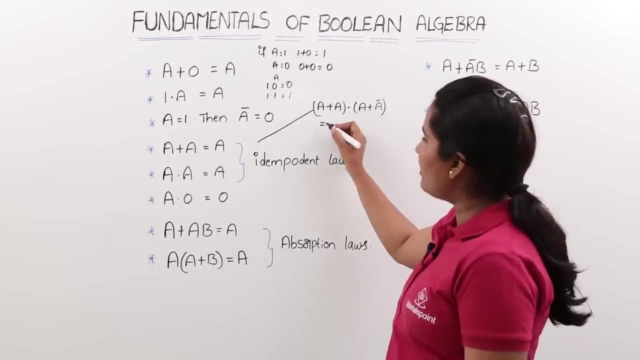 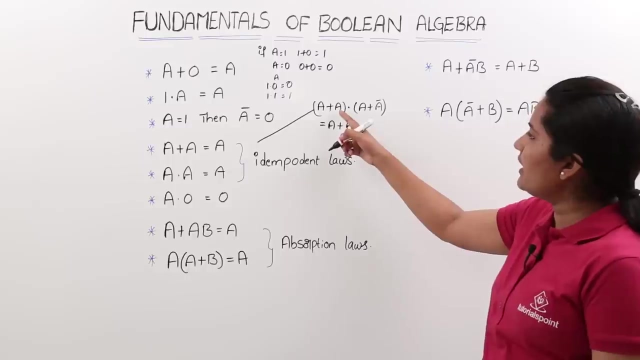 taking a plus a into a plus a bar like this to solve this: here I am just multiplying a into a, So is equivalent to a only Again. a into a Again, equivalent to a only So. next, again, a into a bar is equivalent to 0.. Again a into a bar. 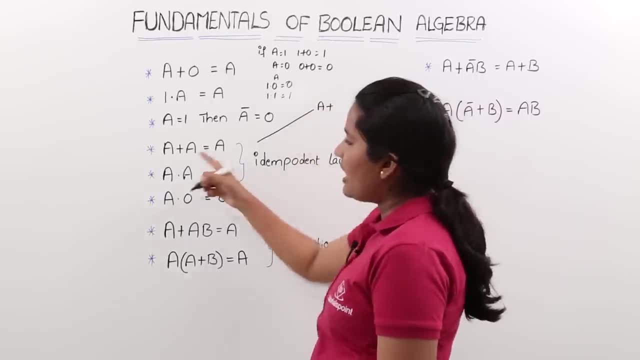 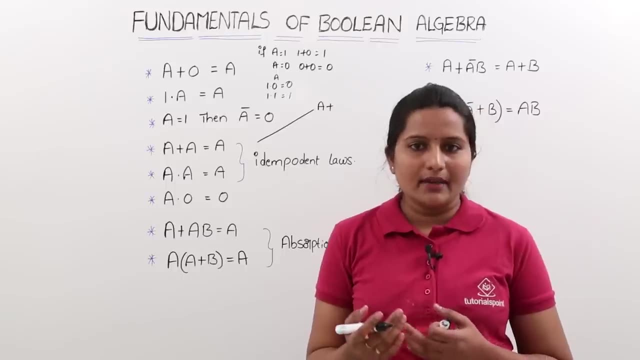 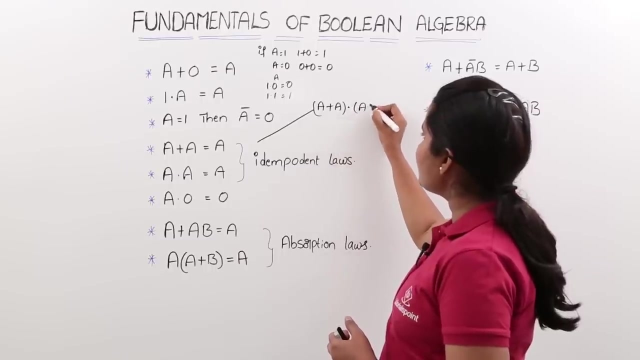 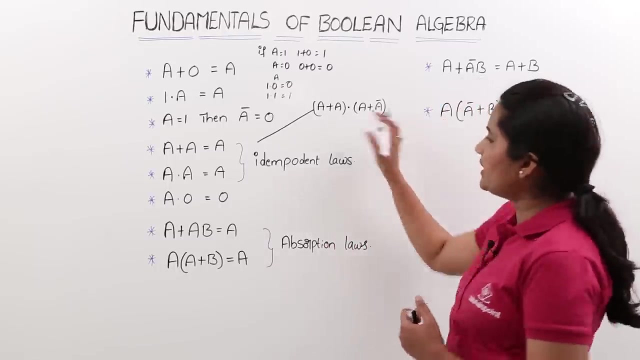 a plus for this a. I can take a plus a bar also. For example, if you are having a plus a here, I am just considering into 1.. Into 1 means a plus a bar I can take. a plus a bar is equal to 1. because so here a plus a bar means, for example, a is equal to 0, definitely a bar is. 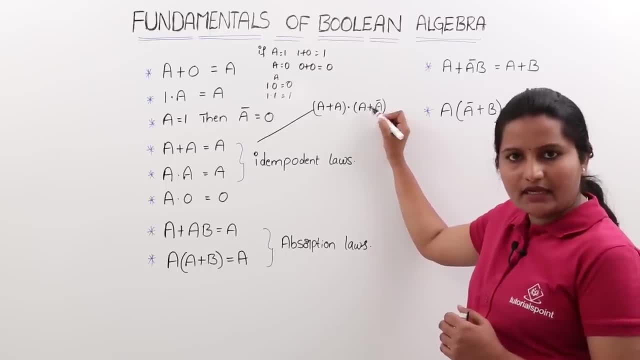 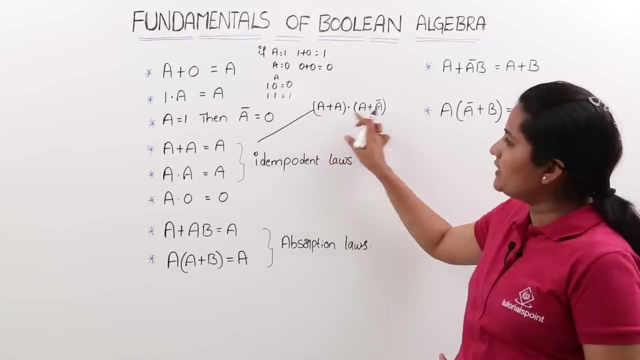 1. If a bar is 1, if a is 1, a bar is 0.. In any case of a, the value is equal to 1.. So if I multiplied anything with 1, we are getting same thing by using this. So that is why I. 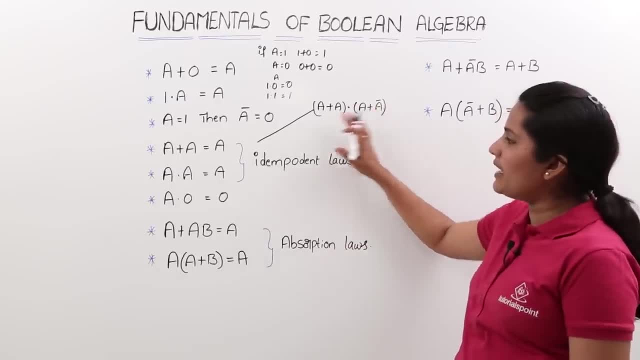 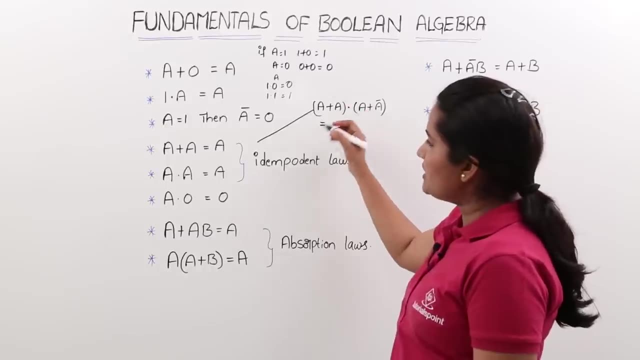 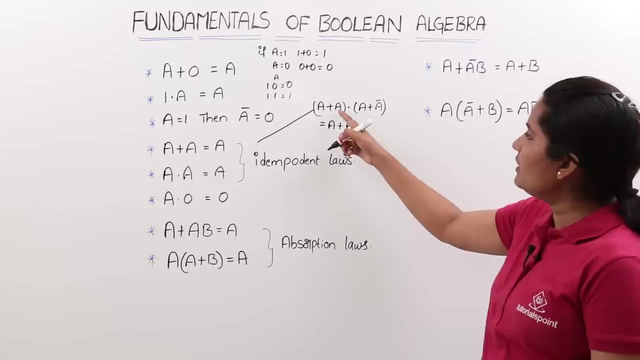 am just taking a plus a into a plus a bar like this to solve this: here I am just multiplying a into a, So is equivalent to a only Again. a into a Again equivalent to a only So. next, again, a into a bar is equivalent to 0.. Again, a into a bar. 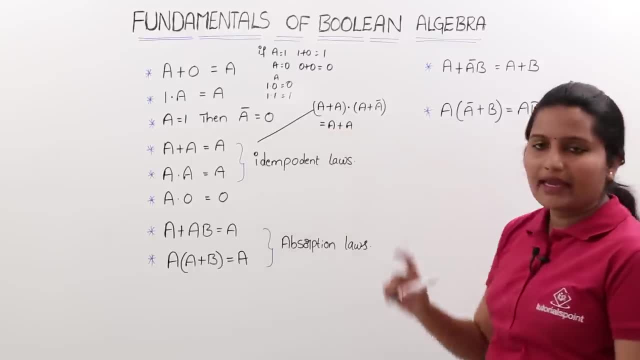 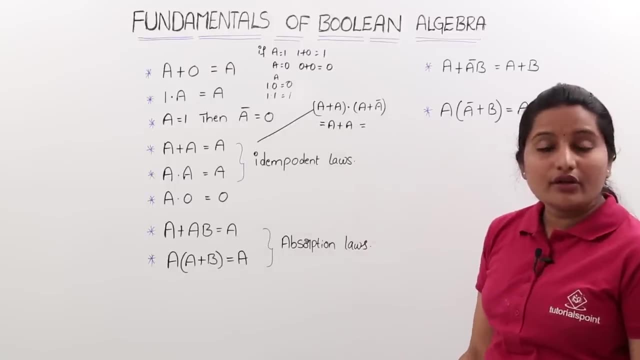 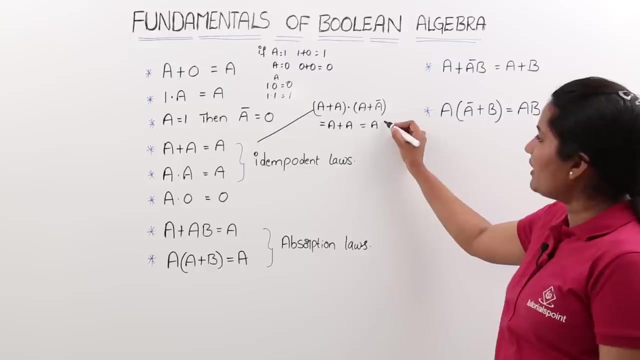 is equivalent to 0.. So now you are getting a plus a. When you are getting a plus a, you can take common of a, So you can have 1 plus 1 there. So that means again, you are getting a plus a, So you can take common of a in this 2. You are getting 1 plus 1.. 1 plus 1. Logical. 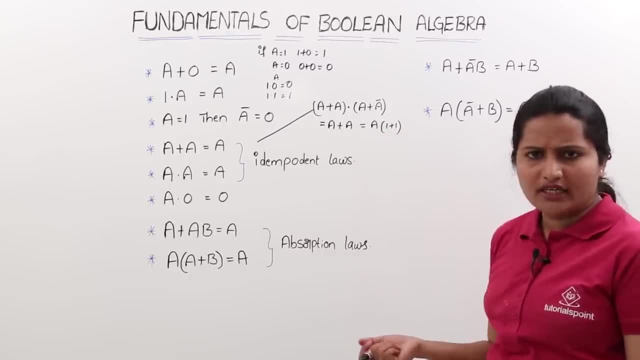 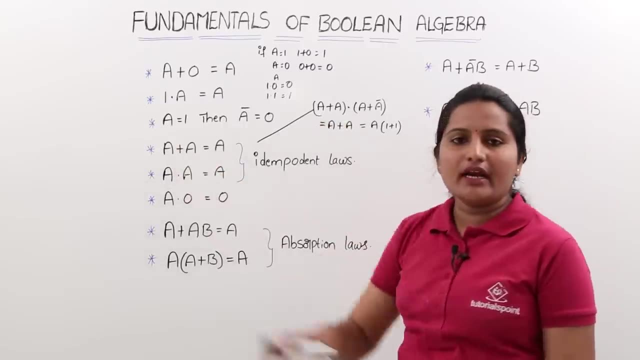 1 plus 1 is equivalent to 1, only a into 1 means a again, So now no need to take this also By. here itself you can take common of a, So you are having 1 plus 1.. So you are. 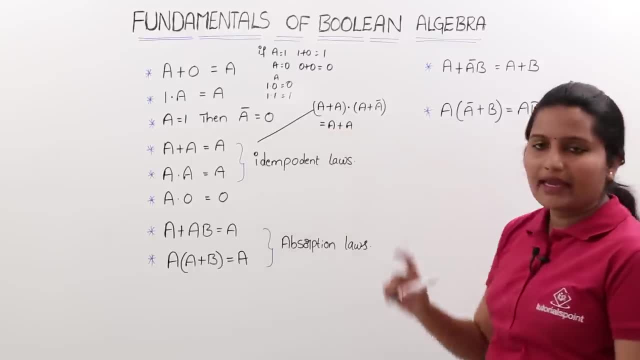 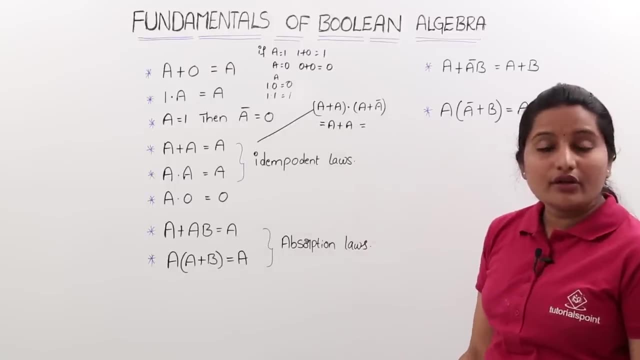 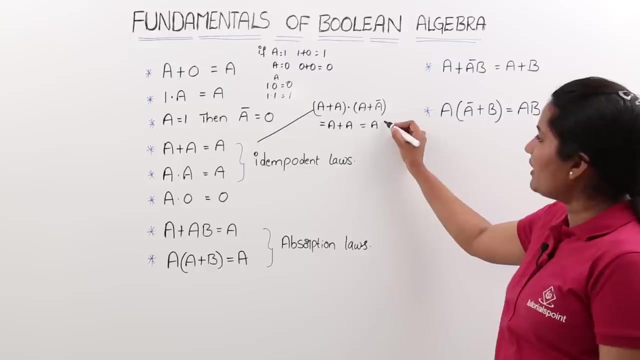 is equivalent to 0.. So now you are getting a plus a. When you are getting a plus a, you can take common of a, So you can have 1 plus 1 there. So that means again you are getting a plus a, So you can take common of a. in this two You are getting 1 plus 1.. 1 plus 1.. Logical. 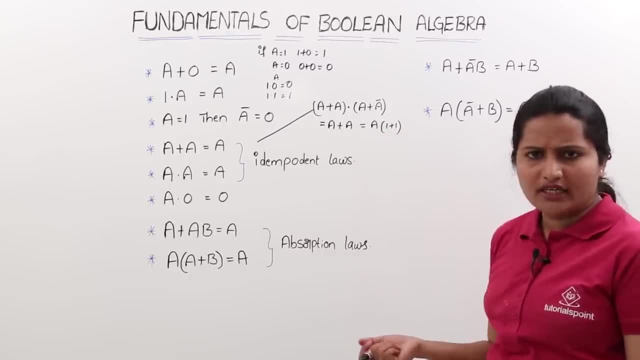 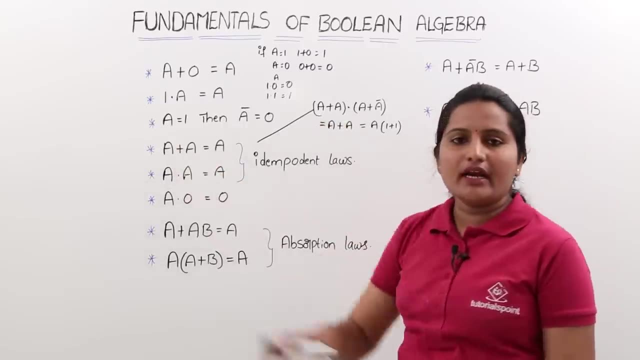 1 plus 1 is equivalent to 1, only a into 1 means a again, So now no need to take this also By. here itself you can take common of a, So you are having 1 plus 1.. So you are. 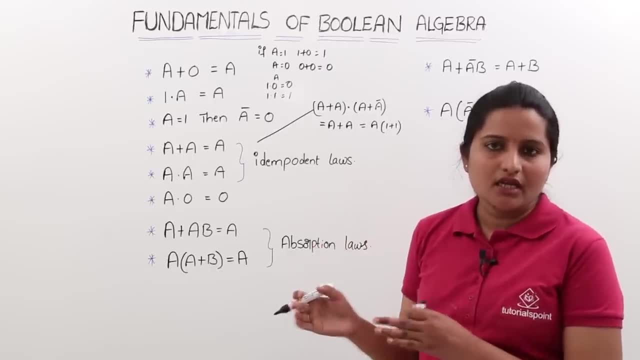 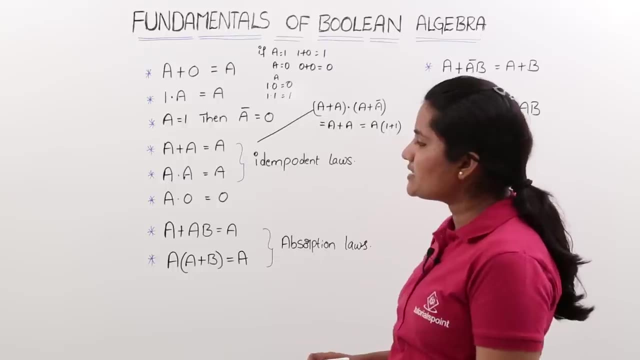 having 1 plus 1.. When you are having logical 1 plus 1, the value is 1.. 1 into a is equal to again a like this: Now you can take: a into a is equal to a. a into a is equal to a means. 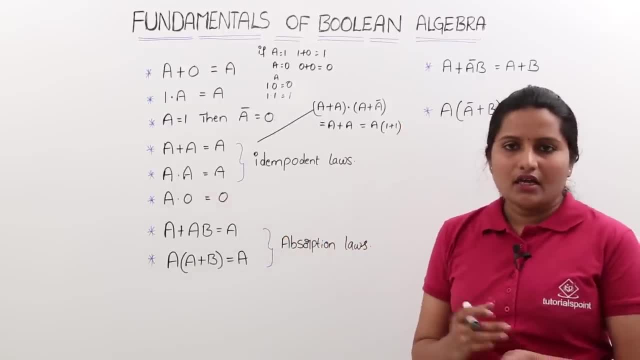 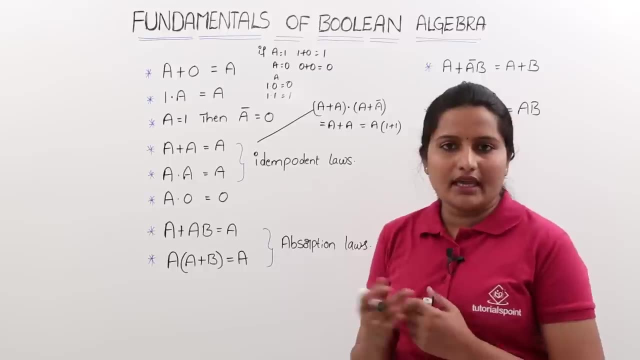 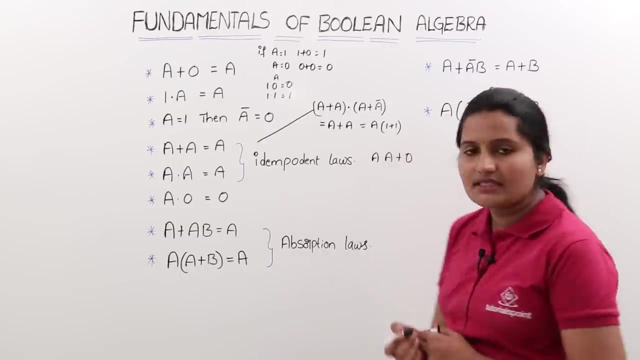 here also you are having one equation That means you can take a into a, So into a into a bar. You can take like this To solve this: a into a. I am adding a 0 here. Is there any difference? By adding 0 to the LHS? Is there any difference? 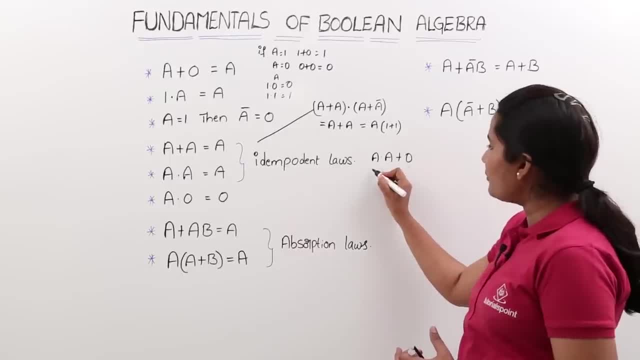 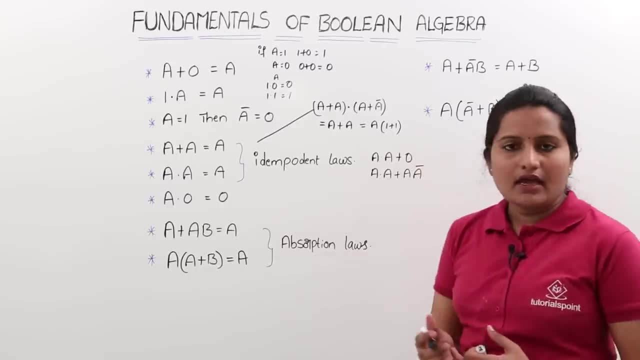 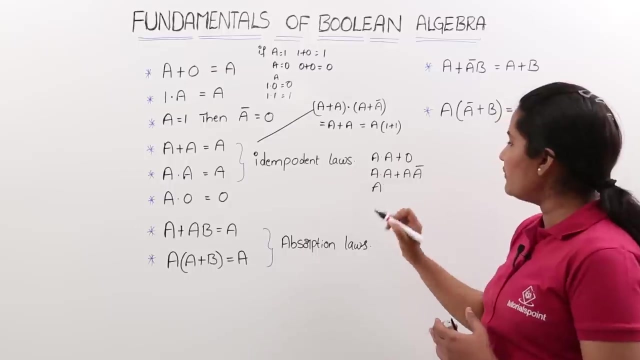 No difference, right? So for this 0 I am going to add a into a plus a into a bar. So 0 is I am taking like a into a bar. Now see, here we can take common of a here. So if you take, 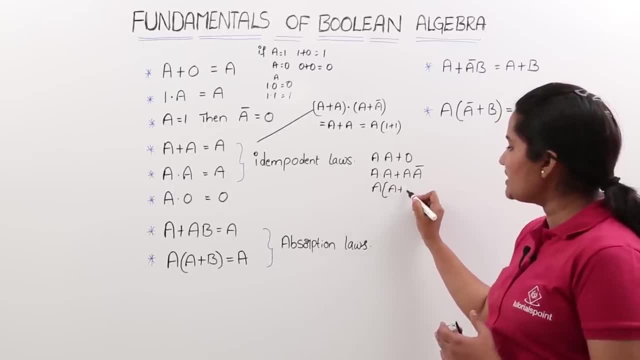 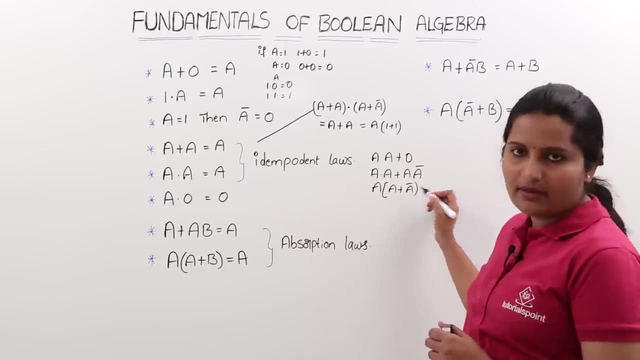 a common of a. what you are getting means a plus a bar. Again, a plus a bar is equivalent to 1 here, because if a is 0, a bar is 1.. If a is 1, a bar is 0.. So like that, in any way, in any case of a, this value is equivalent to 1.. So this: 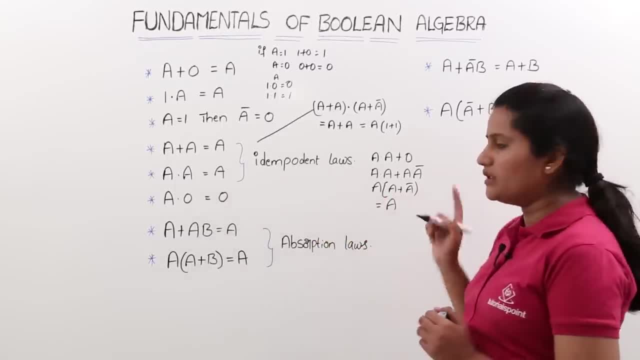 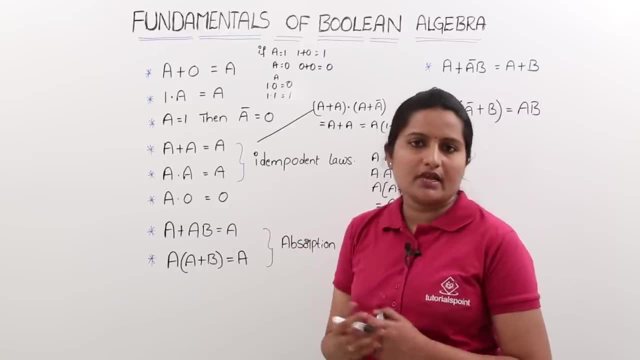 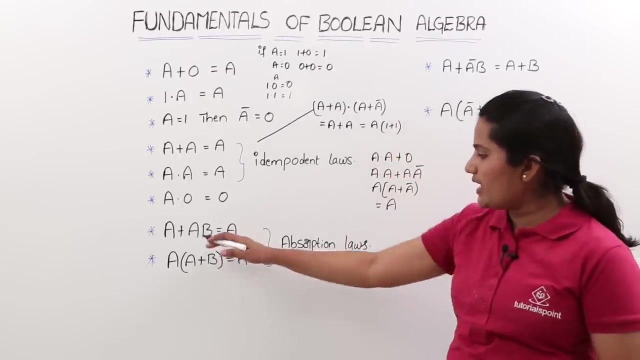 is equivalent to a. So like this we can solve this. Similarly, a into 0 is equal to 0.. This is another fundamental we can use by solving Boolean expressions. When anything multiplied with 0, that will reflect 0. only Next we are having absorption loss, like a plus ab is equal. 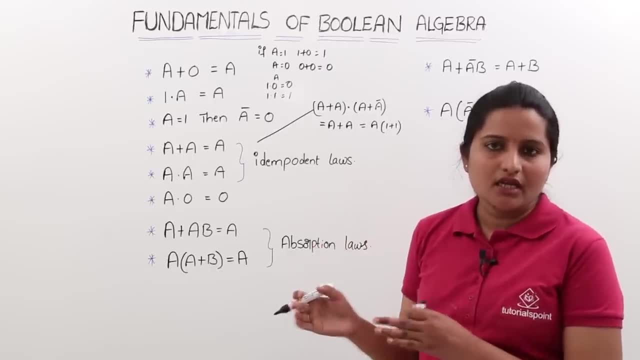 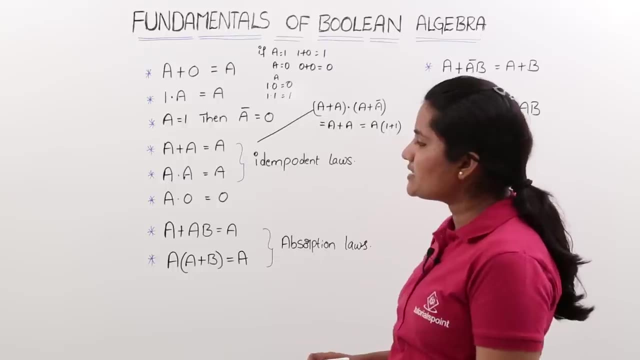 having 1 plus 1.. When you are having logical 1 plus 1, the value is 1.. 1 into a is equal to again a like this: Now you can take: a into a is equal to a. a into a is equal to a means. 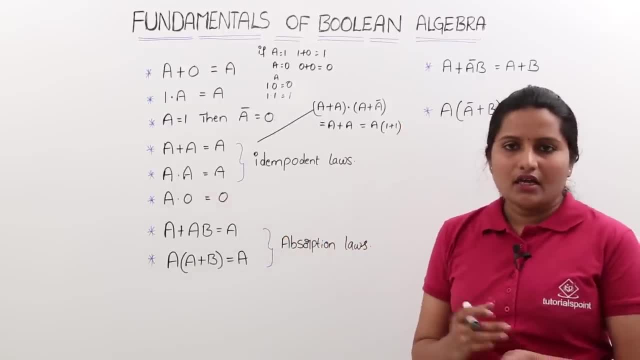 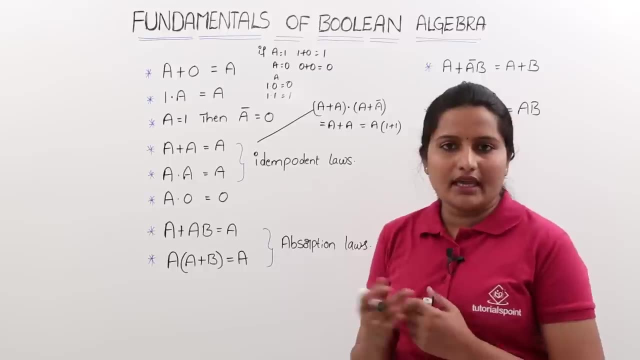 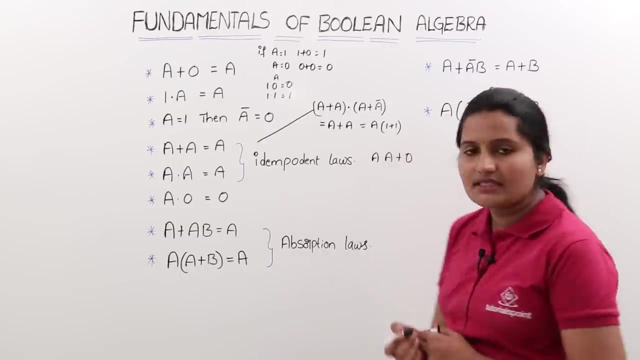 here also you are having one equation That means you can take a into a, So into a into a bar. You can take like this To solve this: a into a. I am adding a 0 here. Is there any difference? By adding 0 to the LHS? Is there any difference? 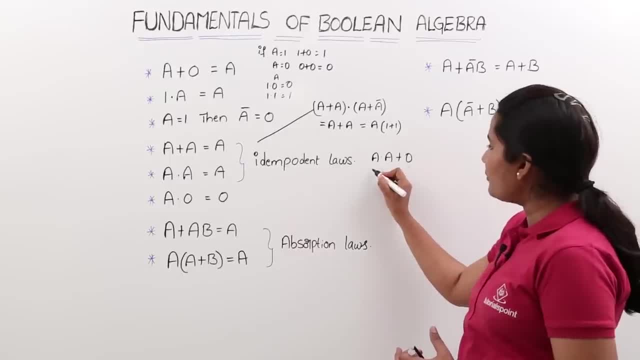 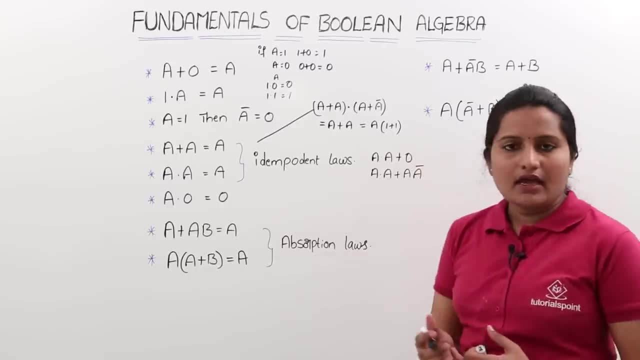 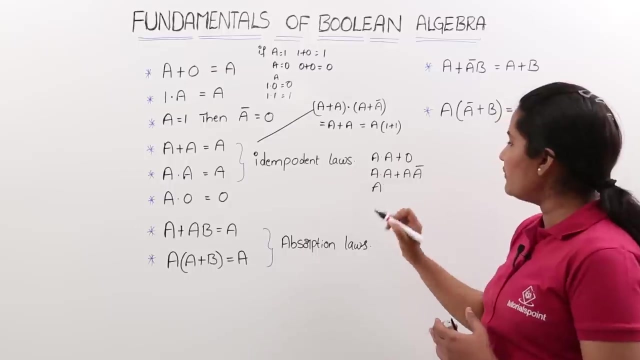 No difference, right? So for this 0 I am going to add a into a plus a into a bar. So 0 is I am taking like a into a bar. Now see, here we can take common of a here. So if you take, 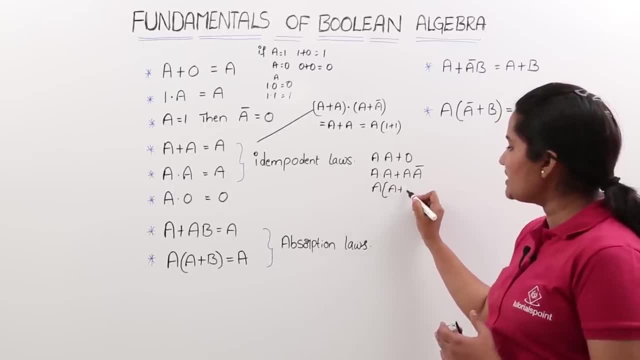 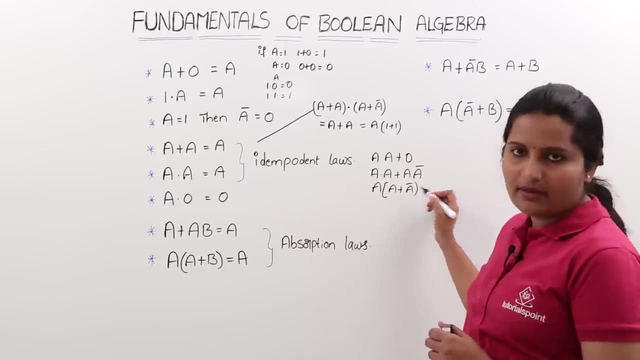 a common of a. what you are getting means a plus a bar. Again, a plus a bar is equivalent to 1 here, because if a is 0, a bar is 1.. If a is 1, a bar is 0.. So like that, in any way, in any case of a, this value is equivalent to 1.. So this: 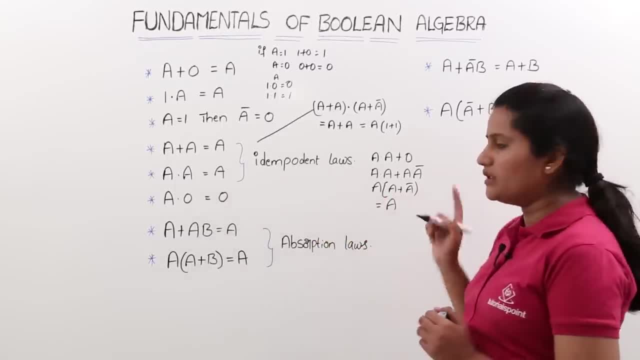 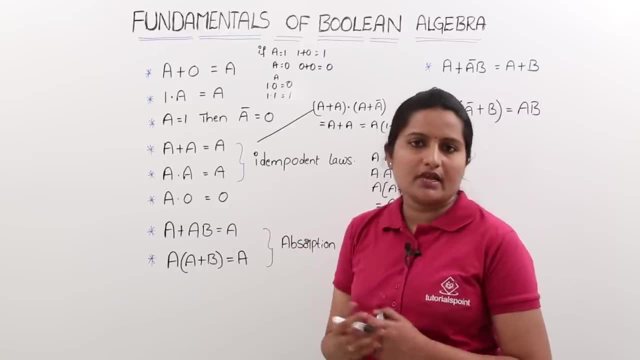 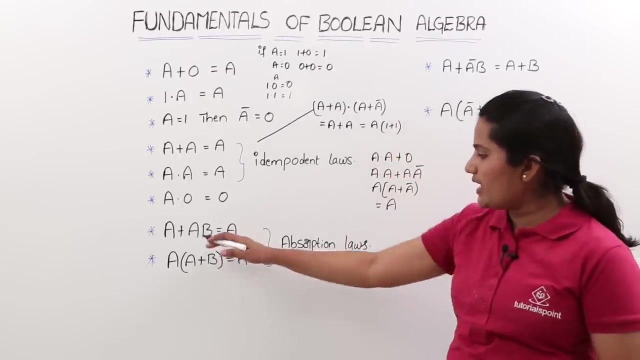 is equivalent to a. So like this we can solve this. Similarly, a into 0 is equal to 0.. This is another fundamental we can use by solving Boolean expressions. When anything multiplied with 0, that will reflect 0. only Next we are having absorption loss, like a plus ab is equal. 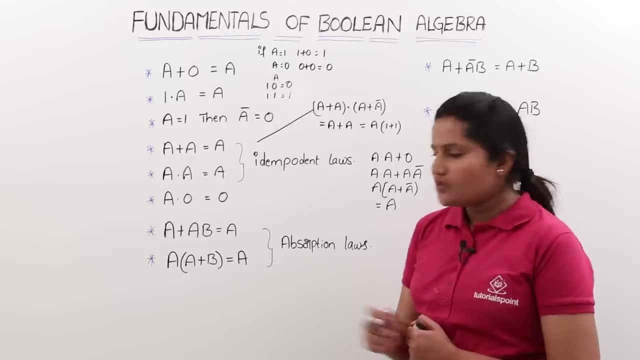 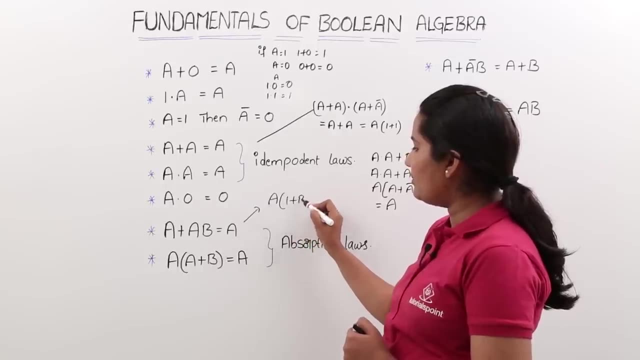 to a. a into a plus b is equal to a. So here you can just take common of a. So that means a into 1 plus b will come. So this is equivalent to 1 plus anything, 1 plus 1.. For example if 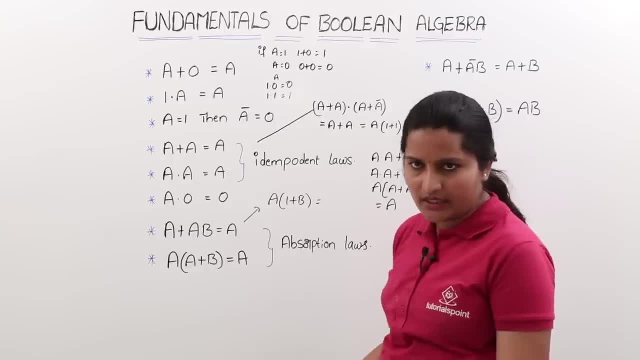 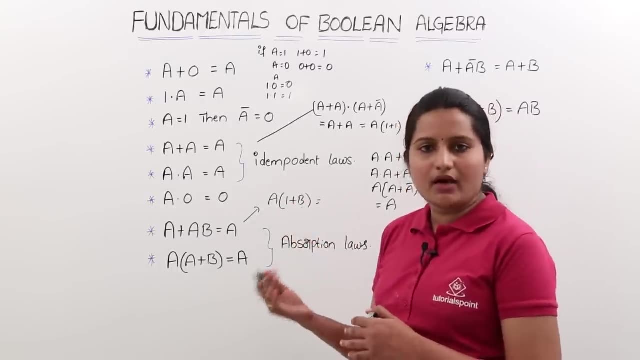 b is equal to 1, 1 plus 1 is equal to 1 only If b is equal to 0, 1 plus 0 is also 1.. So a is multiplied with 1 always. So definitely the value is equivalent to a here. 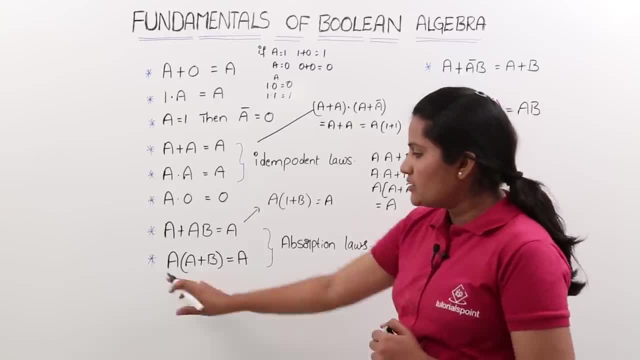 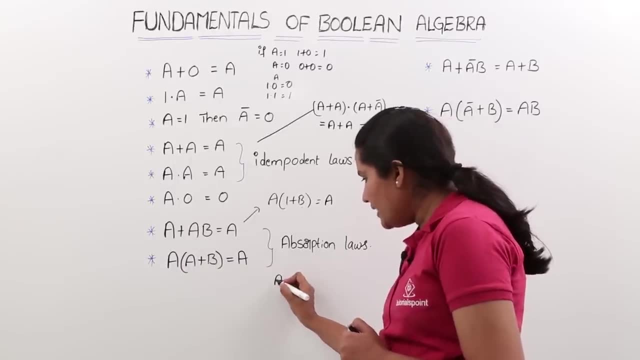 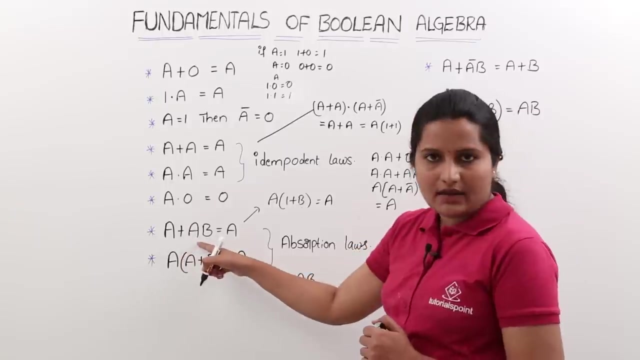 So in the same way. so see this second absorption law. So here a into a is equal to. I am just multiplying to inside. a into a is equal to a. Next place: a into b is equal to ab. So here this is nothing but this law. So definitely this is equivalent to a. here I am just multiplying. 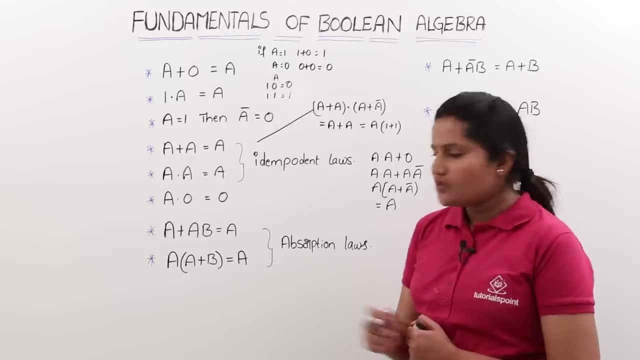 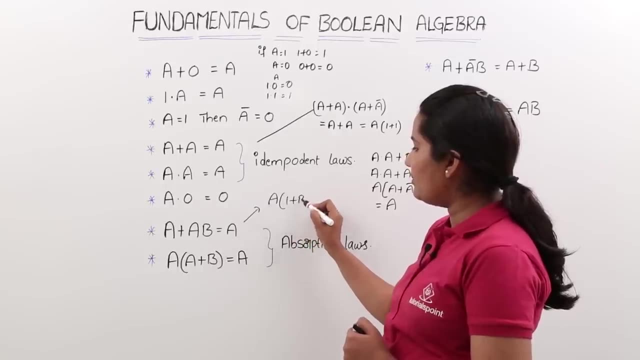 to a. a into a plus b is equal to a. So here you can just take common of a. So that means a into 1 plus b will come. So this is equivalent to 1 plus anything, 1 plus 1.. For example if 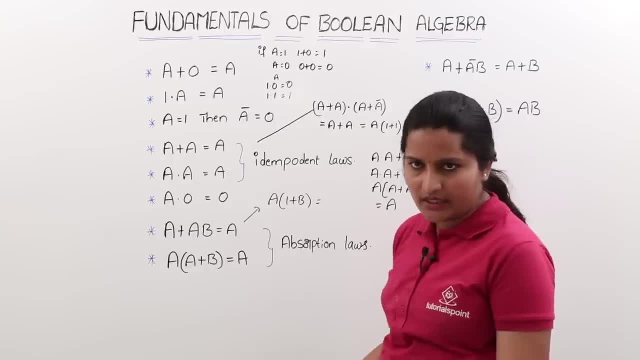 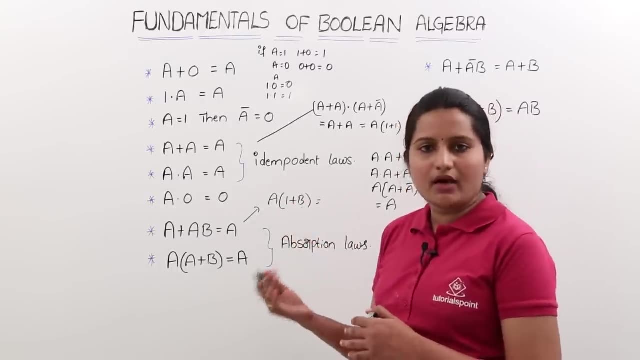 b is equal to 1, 1 plus 1 is equal to 1 only If b is equal to 0, 1 plus 0 is also 1.. So a is multiplied with 1 always. So definitely the value is equivalent to a here. 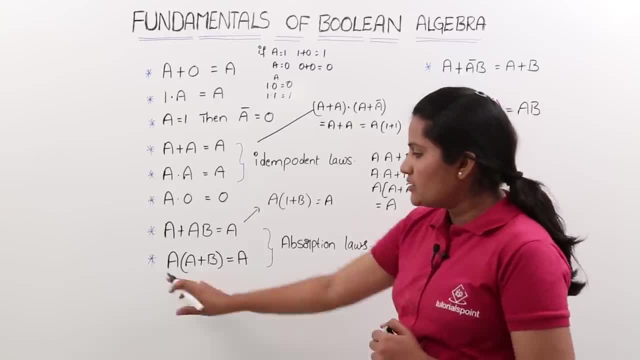 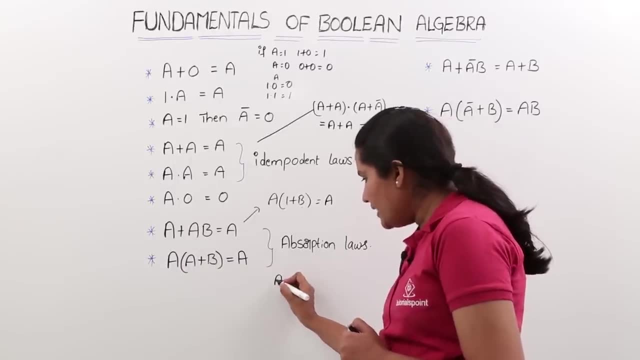 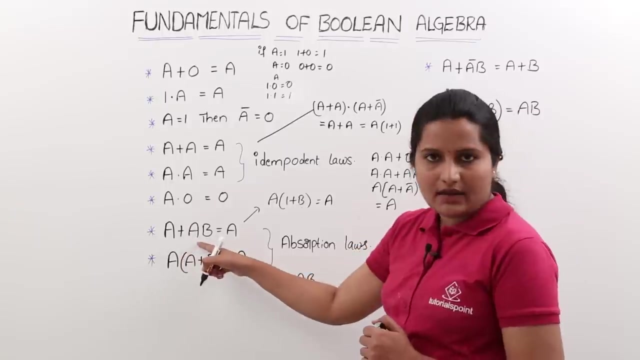 So in the same way. so see this second absorption law. So here a into a is equal to. I am just multiplying to inside. a into a is equal to a. Next place: a into b is equal to ab. So here this is nothing but this law. So definitely this is equivalent to a. here I am just multiplying. 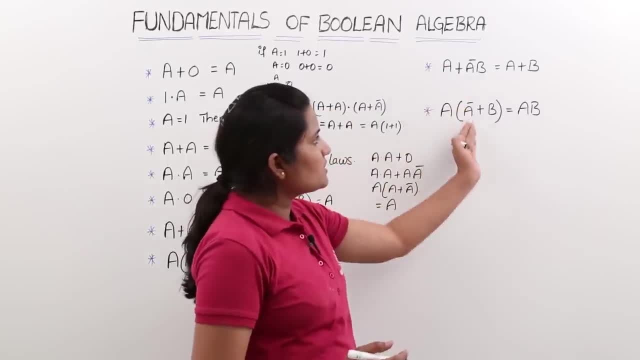 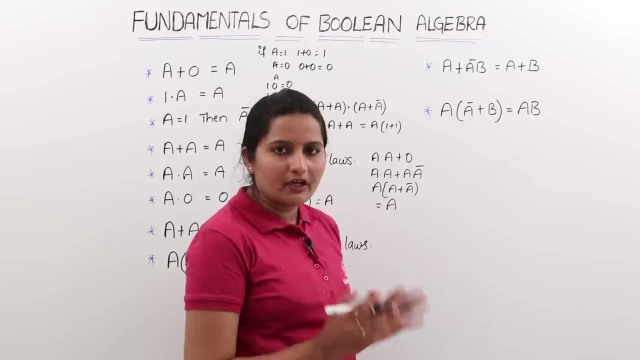 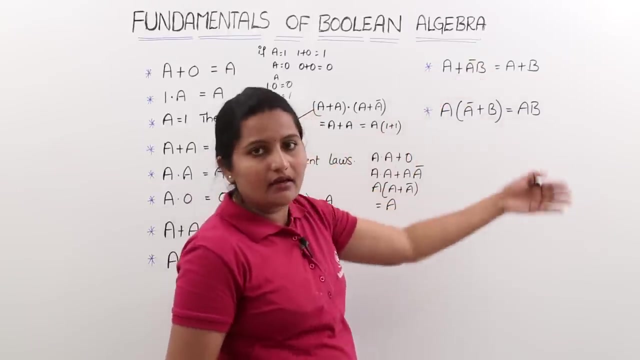 to inside. That is it. So now see here last two fundamentals. This is a plus a. bar b is equal to a plus b. This is very, very important fundamental that you are going to use mostly in Boolean expression solving, And it came directly in gate questions In one of the 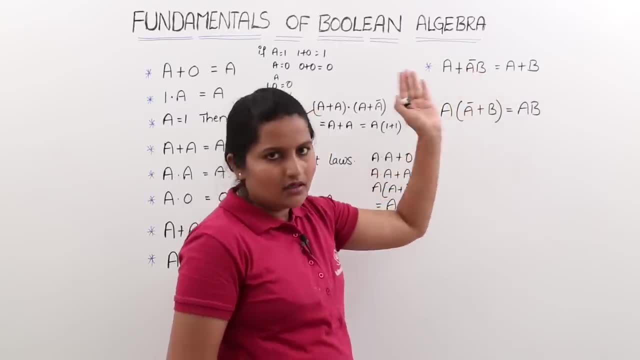 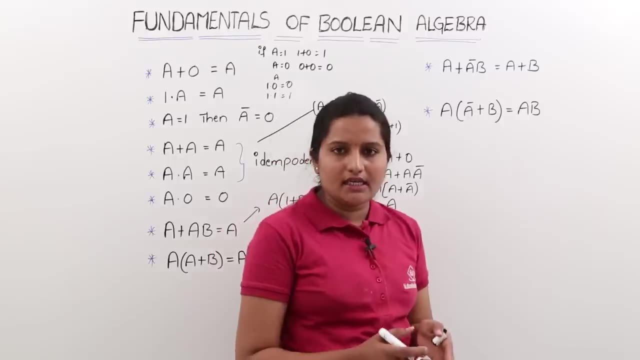 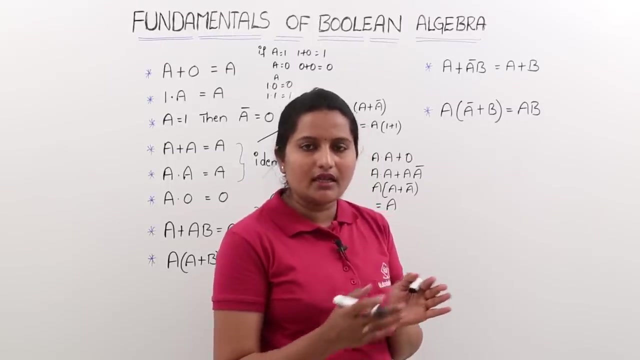 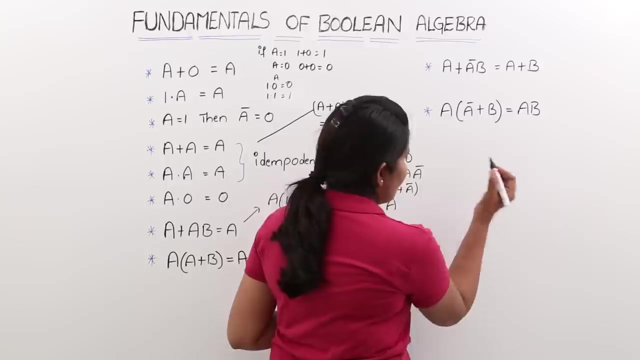 years of gate problems. So it came directly. So what is the value equivalent to a plus a bar b? So that is equal to a plus b. So here what you need to think is anything added with multiplication of its complement and other number, then definitely you are having a plus b. For example, if you are having like, 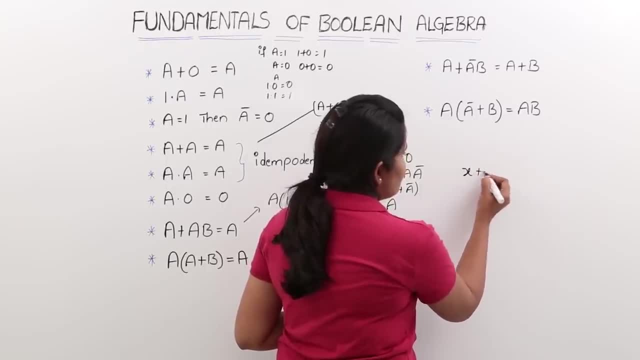 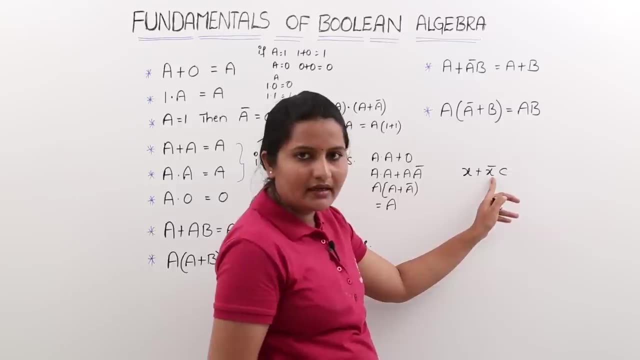 this: that means x plus x bar c, like this: if you saw anywhere For this x, you are having complement here. So this complement multiplied with some other thing, So this is a plus a back. So this is also a x plus c. for example, if you are having like this, It is a plus. a b, so this is a plus c. So in this case of you know, a plus c is equal to a plus a bar and other one the phrasal letter. but the second part of a plus b is x plus a is a. it is x plus x bar. So this is b, it is a plus. you have this completly, So here. 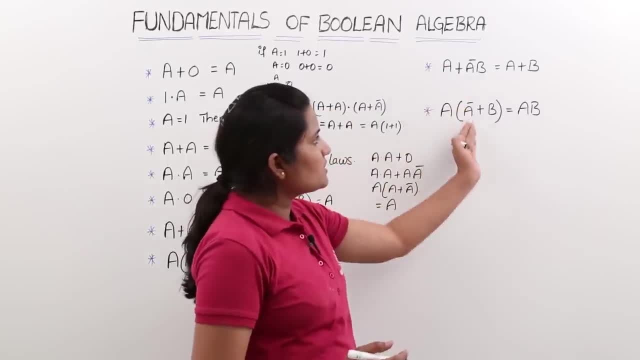 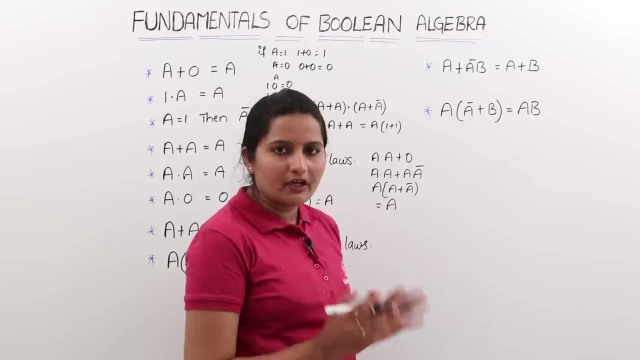 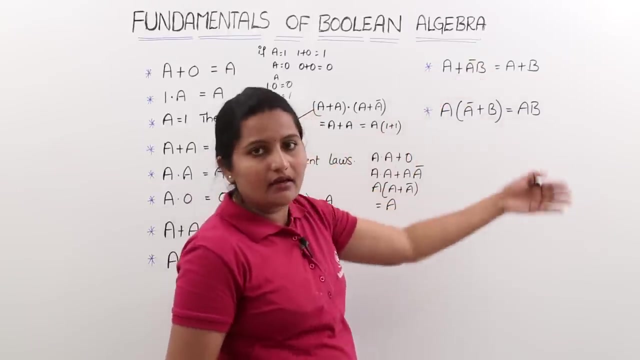 to inside. That is it. So now see here last two fundamentals. This is a plus a. bar b is equal to a plus b. This is very, very important fundamental that you are going to use mostly in Boolean expression solving- And it came directly in gate questions one in one of the 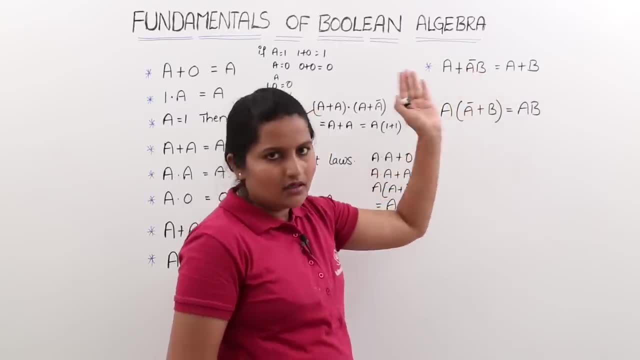 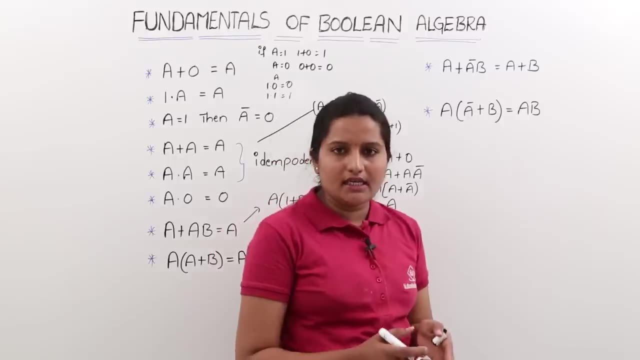 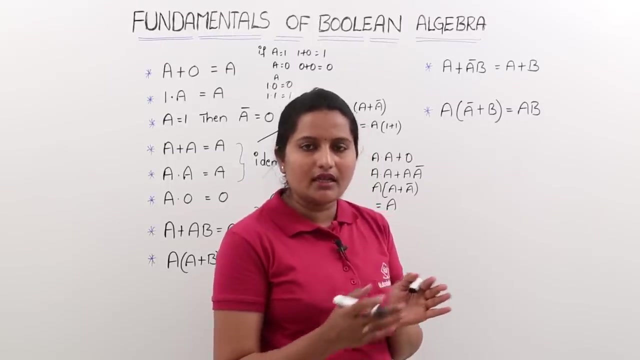 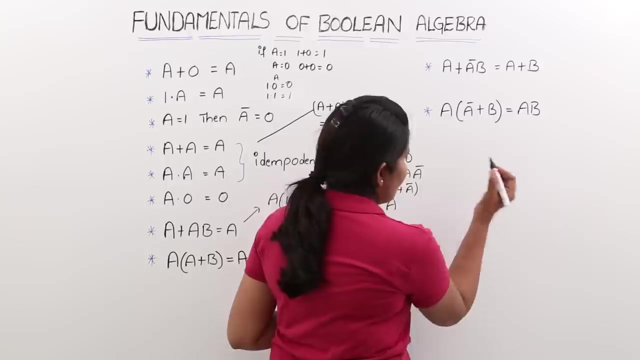 years of gate problems. So it came directly. So what is the value equivalent to a plus a bar b? So that is equal to a plus b Here. what you need to think is anything added with multiplication of its complement and other number, then definitely you are having a plus b. For example, if you are having like, 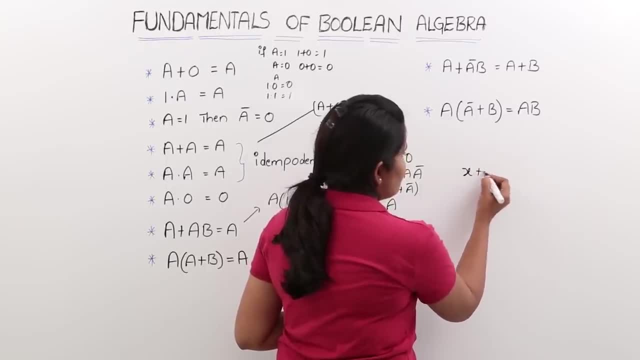 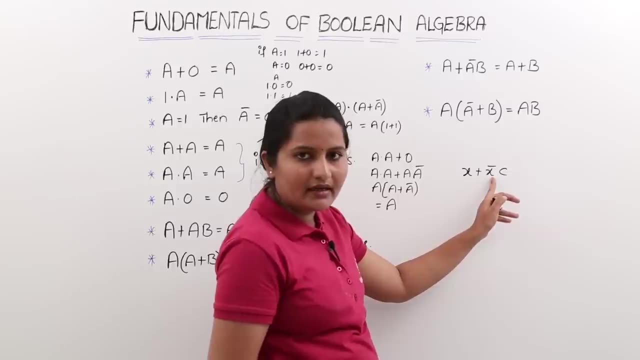 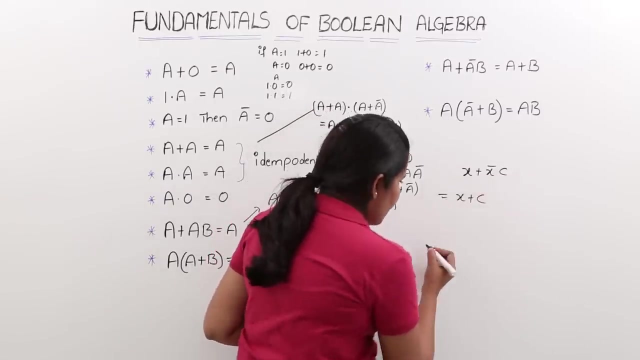 this: that means x plus x bar c, like this: if you saw anywhere For this x, you are having complement here. So this complement multiplied with some other thing, So you can take this as x plus c. for example, if you are having, like this: a plus, c plus. 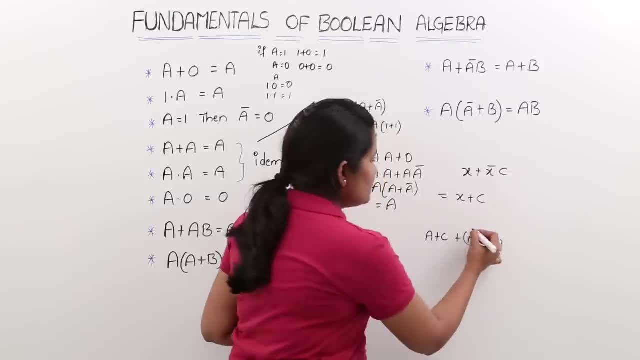 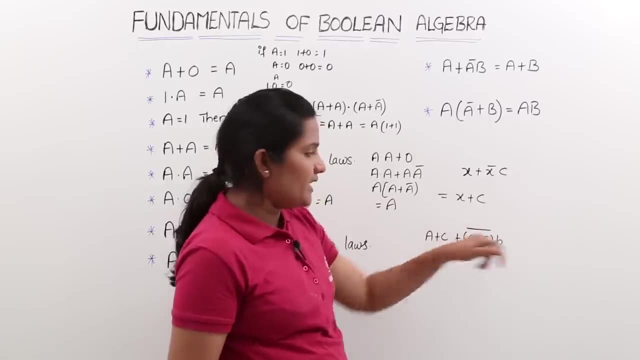 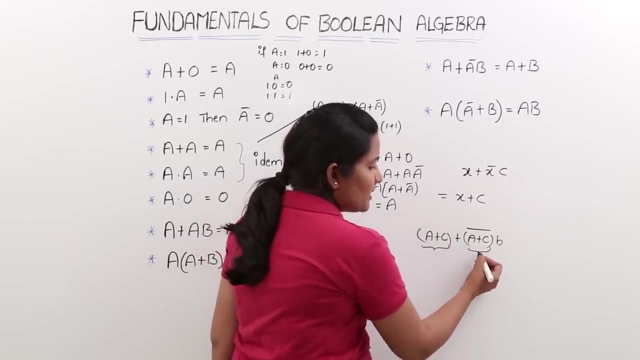 a plus c into b. like this you have an expression a plus c, a plus c, bar into some b is there. So now, here, this is the complement. for this complement, something is multiplied, So now you can take this as a plus c. So next you have capital C equal to a plus c plus b, right, 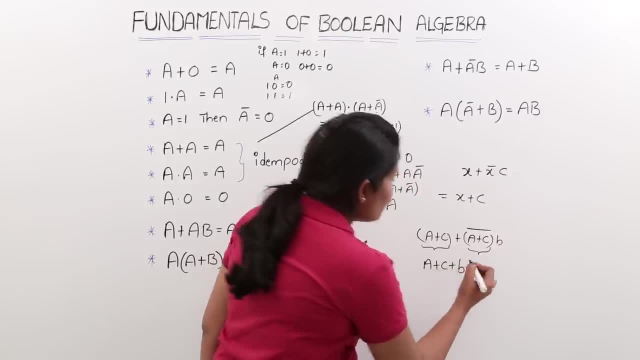 What you have here is a plus c bar into a, into b. the first thing that we have is arrangement. here you have C bar equal to b. Then from there you can make a particular no less than plus c plus b. So you can apply this fundamental like this. So now we can see how we can. 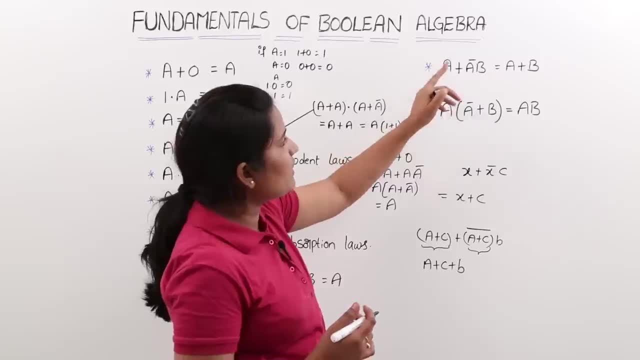 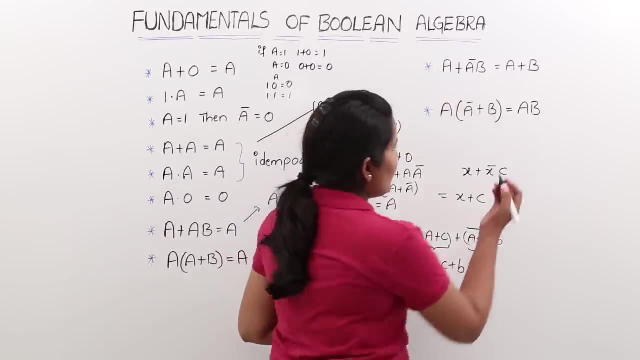 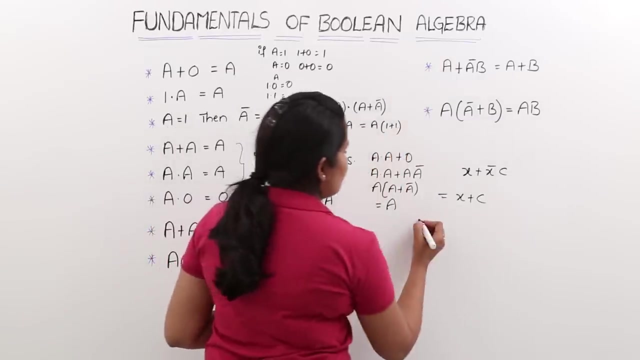 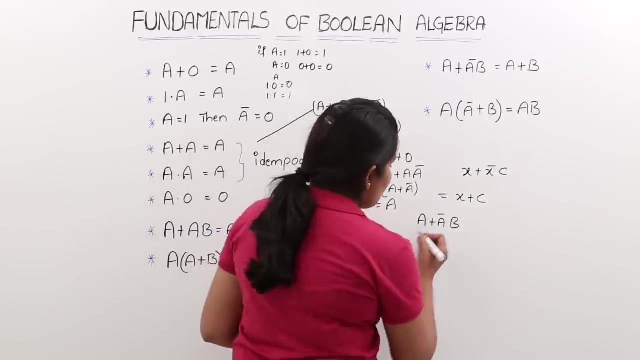 solve this. So I am taking here, I am just adding, I am just multiplying 1 plus b for a to solve that. I am just doing So multiplication of 1 plus b here. see, here I am considering this: a plus a, bar b. I am considering Now for this: I am just multiplying 1 plus b. 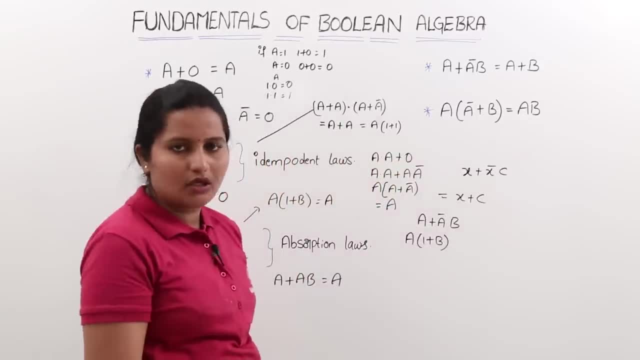 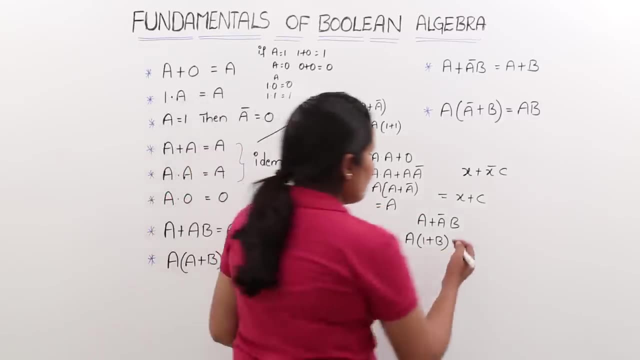 You know the value of 1 plus b. 1 plus anything is equal to 1, only 1 plus some long expression is also 1.. So 1 plus anything is 1 plus a bar b. So now see here a into 1, a next. 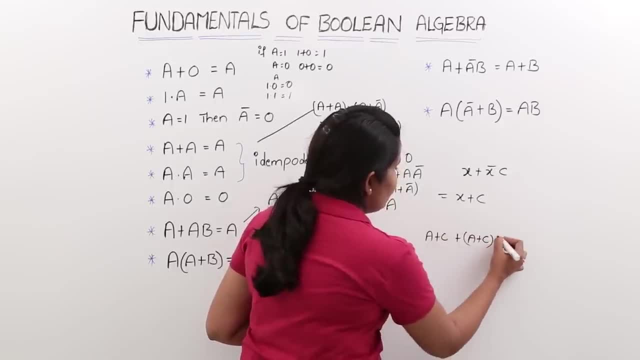 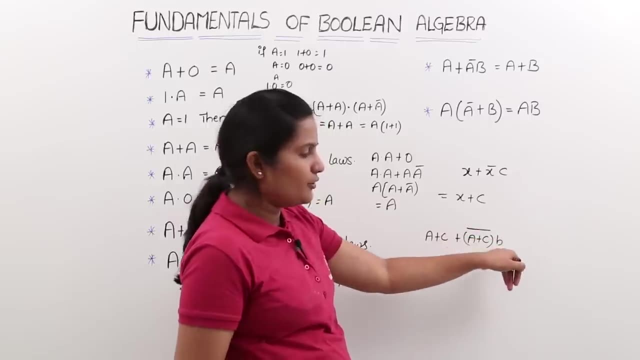 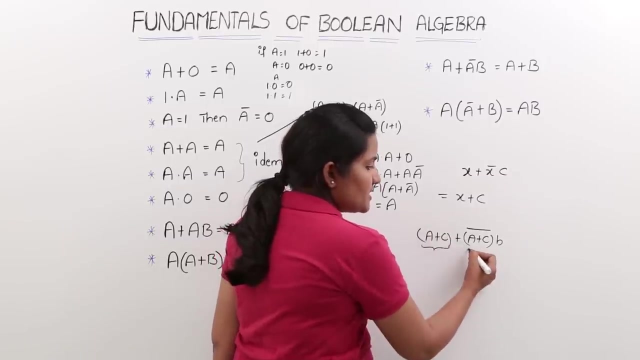 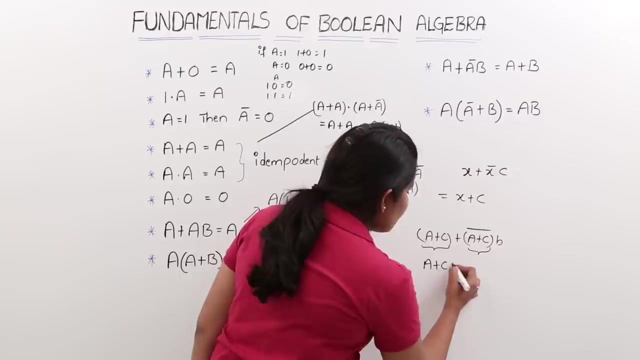 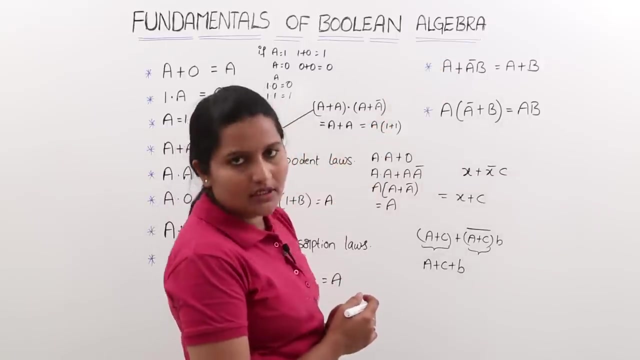 whatever you are. So now you can take this as a plus c plus b, So you can apply this fundamental like this. So now we can see how we can solve this. So I am taking here, I am just adding, I am just 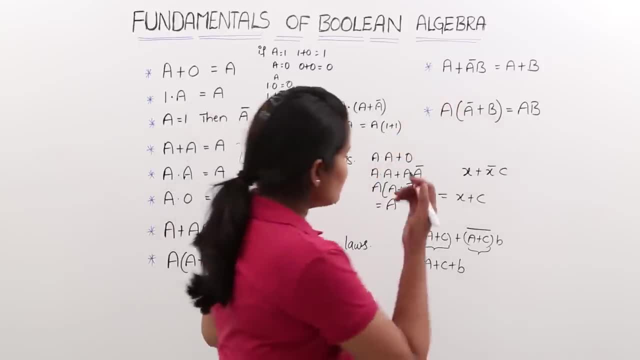 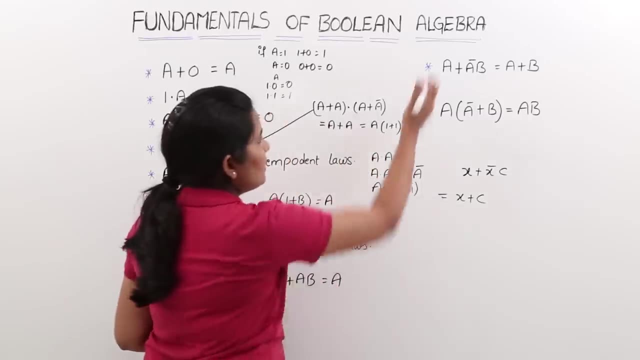 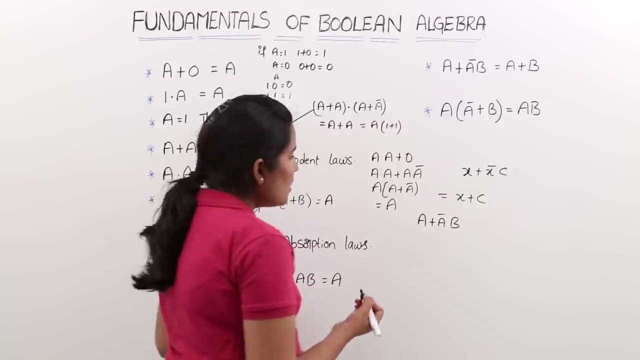 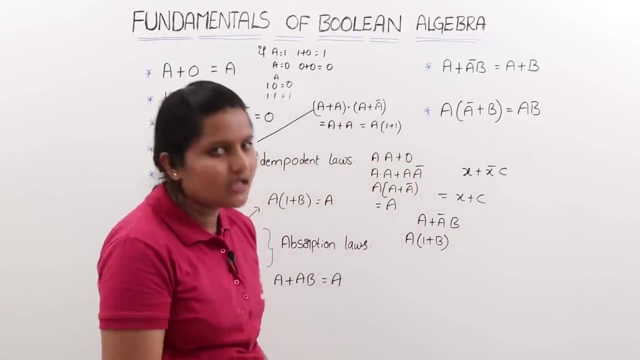 multiplying 1 plus b for a to solve that I am just doing So, multiplication of 1 plus b. here See, here I am considering this: a plus a bar b. I am considering Now for this: I am just multiplying 1 plus b. You know the value of 1 plus b. 1 plus anything is equal to 1 only 1 plus some long. 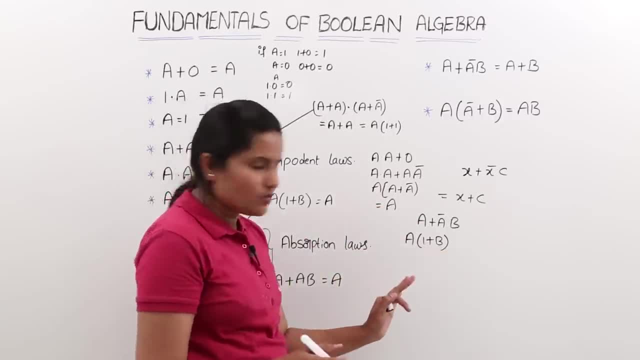 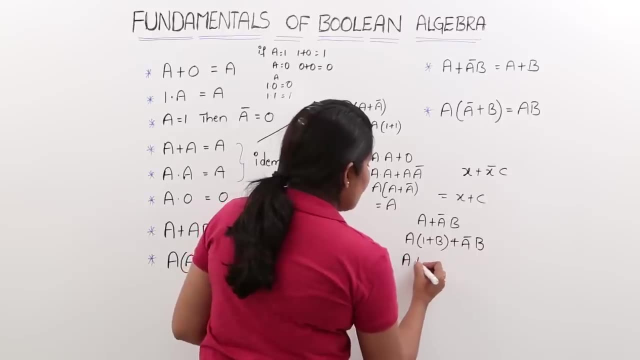 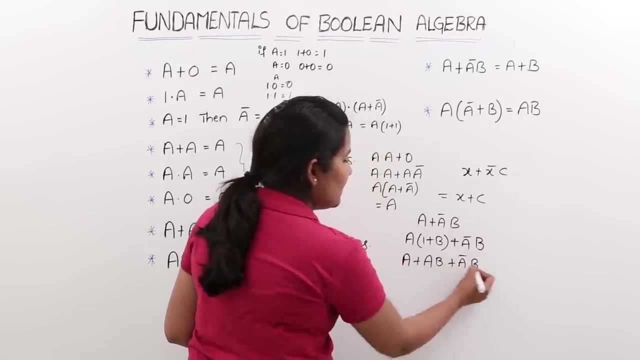 expression is also 1. So 1 plus anything is 1 plus a bar b. So now see here: a into 1, a, next a into b, a, b plus a bar b. Now I am taking common of b in this 2. So now, so here I am taking common. 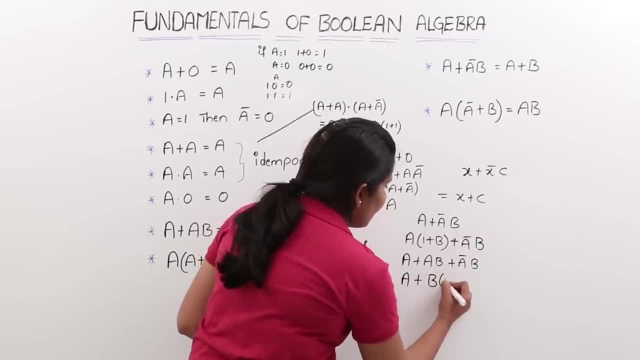 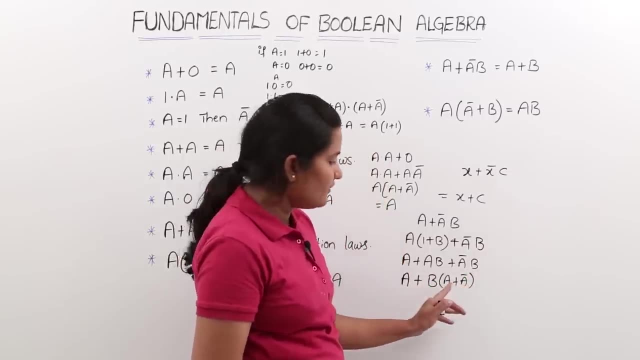 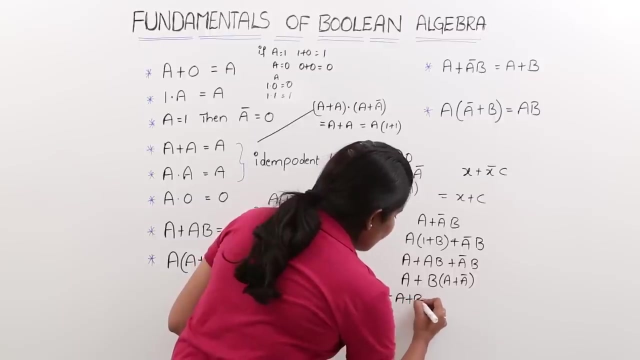 of b, a plus b, into a plus a bar. So here a plus a bar value is equivalent to 1.. You know the value of a plus a bar. So that is equal to 1.. So this is nothing but a plus b. like this We can. 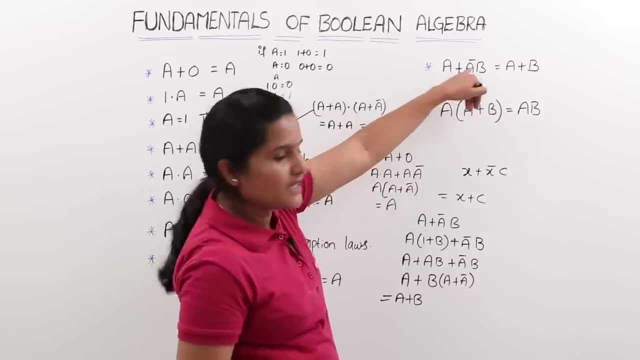 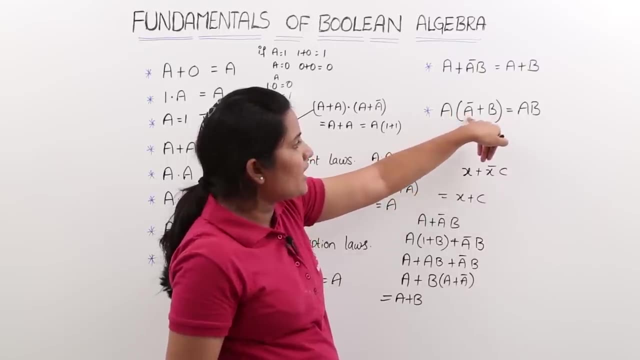 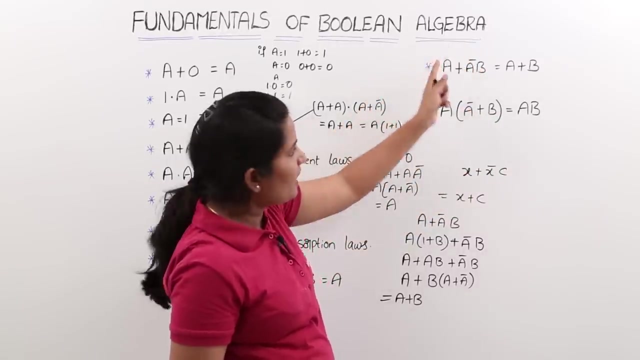 solve this expression. So a plus a bar b is always equivalent to a plus b. In the same way here also see a into a bar plus b is equal to a b. We can, we can say this is dual of this expression. Whenever you are having plus, you are getting multiplication, and whenever you are, 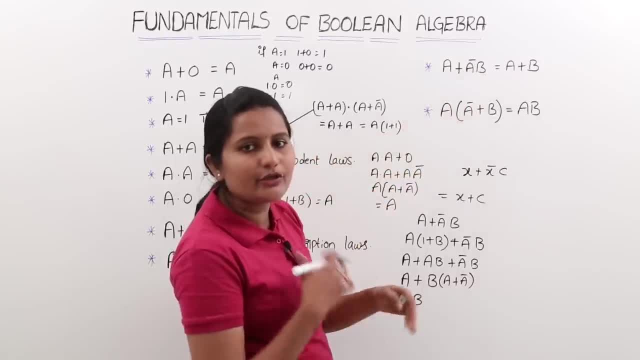 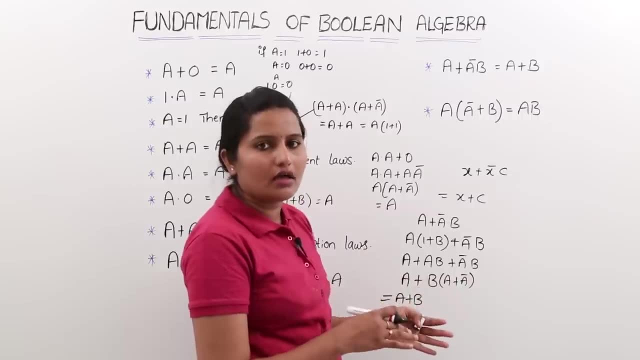 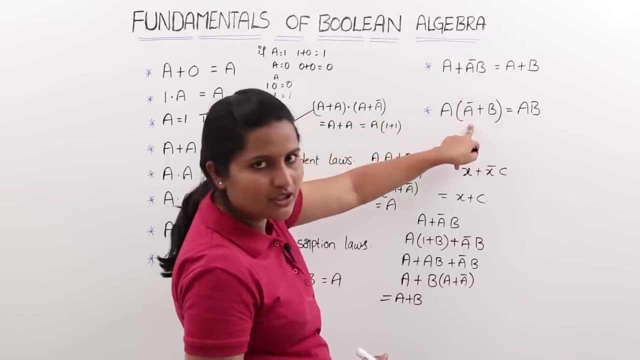 having multiplication. there you are getting plus. This is nothing but dual of expression. Dual means or, Or converted into and and converted into or Plus into multiplication, multiplication into plus. So now, here you are having dual of this expression. So simply, these are this expression.